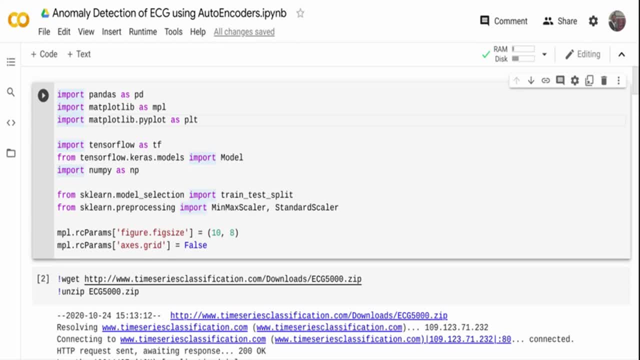 you can click the link on the top, But for this video that is not mandatory. I'll be covering the key aspects of autoencoder in this video itself, But if you want to know more than what I cover in this video, you can use the link on the top or 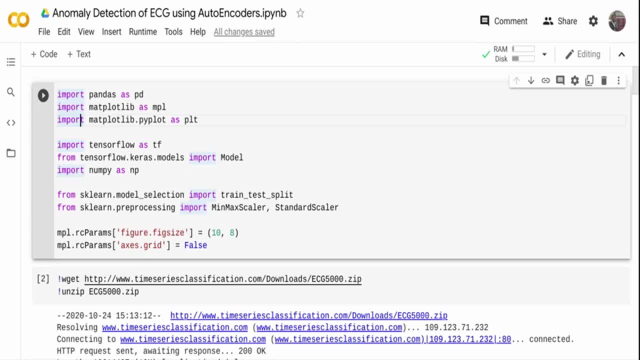 link in the video description to watch details of autoencoder. Now let's get started. So what I'm going to do is I'm importing the typical packages: pandas for reading the data set, matplotlib for visualizing the data set, TensorFlow for 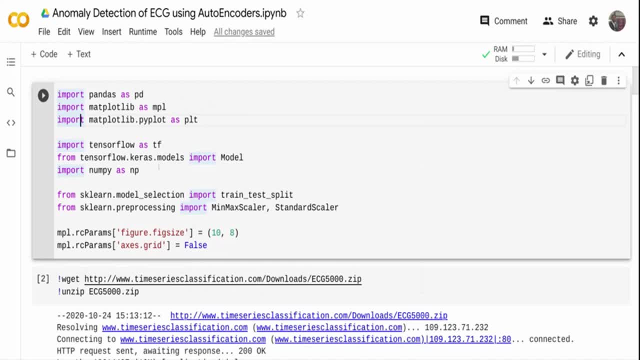 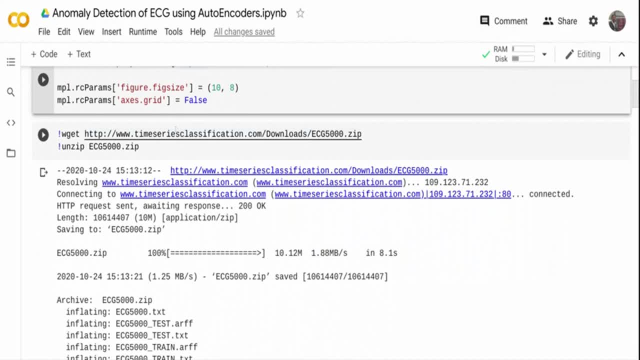 ECG 5000 data set. The data set is available in this particular website, time-serious-classificationcom. You can find a lot of time-serious data set over there. I'm downloading the ECG 5000 data set Now. we all know ECG stands for. 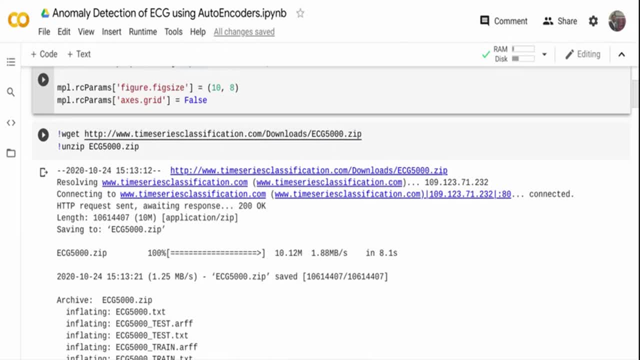 electrocardiogram. Now what this data set is basically. now, first, electrocardiogram: what it is is basically it checks how your heart is functioning by measuring electrical activity of the heart. Now what happens? in each heartbeat, An electrical impulse travels through the heart that creates muscles to squeeze and 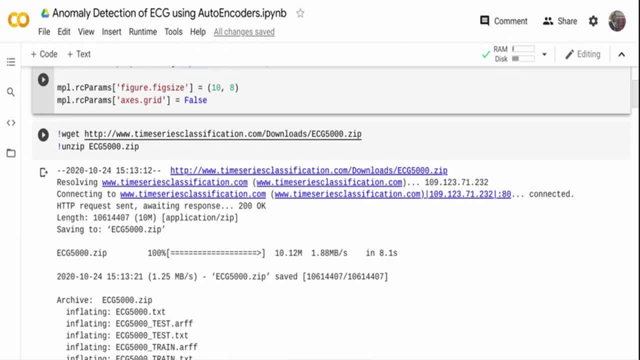 pump blood to the heart. That's what it does, That's what typically our body functions. Now this electrocardiogram: it captures that electrical impulse and that can help doctors determine if the heart function is normal or irregular. So that's what basically an 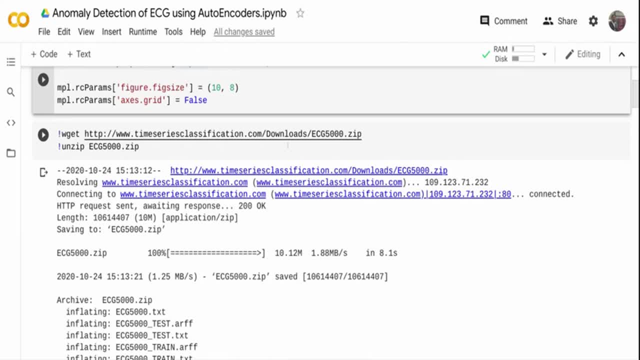 ECG does, And this data set contains information of both the normal activity of the heart and regular activity of the art. and what we are going to do is we are going to take this data set and we are going to build an anomaly detector. right, i already downloaded the data set it might take. 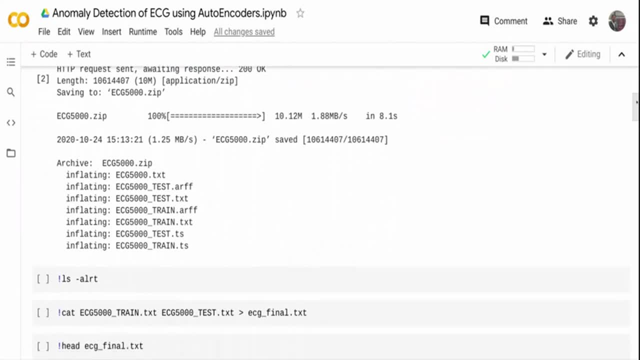 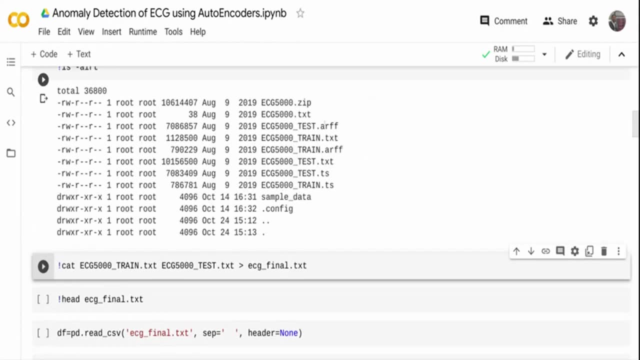 some time, so that's why i already downloaded it. now, if you see the output of this particular download, there are multiple files over here, so there is like an arf file or there's a txt file and there's a dot. here there's a different format of the same file. i'm going to use the dot txt file. 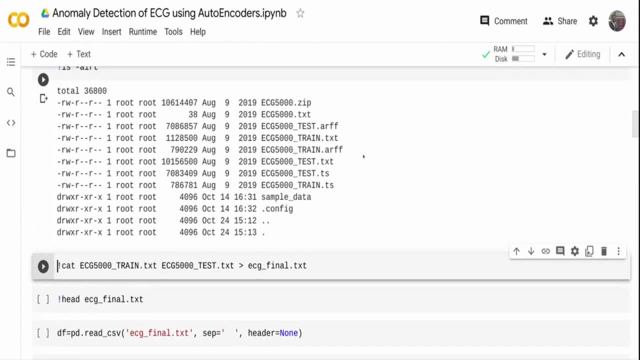 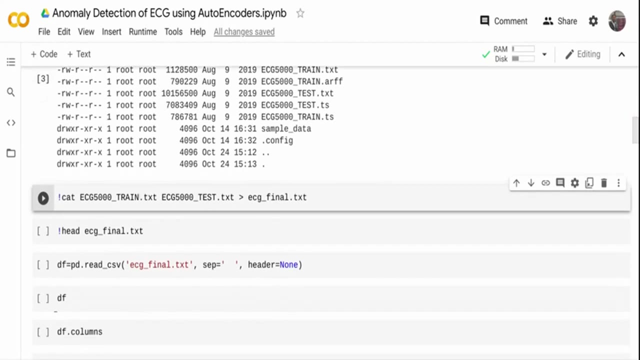 there is a train and test. the train and test combine together makes around 5000 observations. so there are 5000 observations containing both normal activity of the art and irregular activity of the heart right. that's the ecg data set. so what i'm doing is i'm concatenating both. 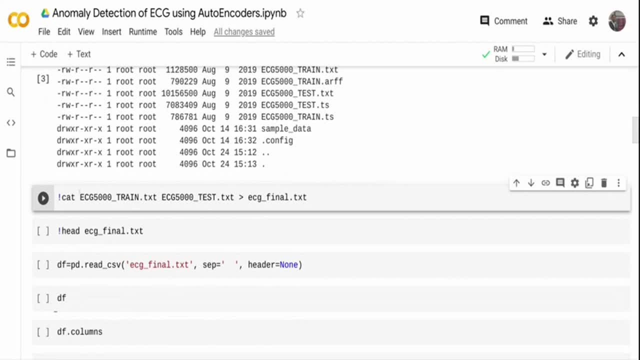 the train and test data set into a single data set. so i'm using an unix function over here, cat. so cat will just like take this to data set. it will display it, but what i'm doing is, while it's displaying and sending the output data, it found that it cannot be saved on the air, which is an. 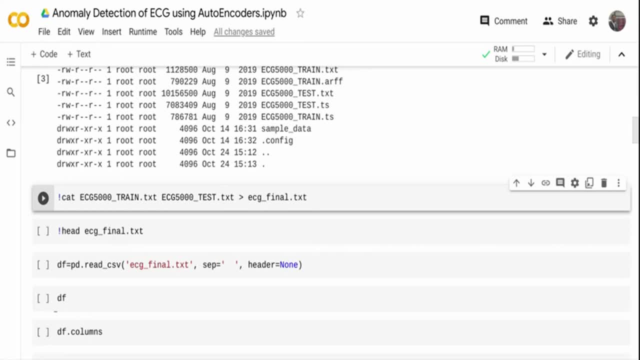 error value. we are distributing choke for free service. and then, what i also value, this data set is gonna be used in the data set. so the Memory Datarow that I have here now is doing an earlier ranking output to another file so that it looks like more a concatenated single file. 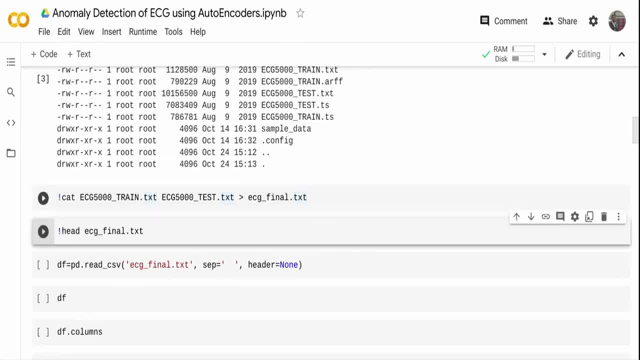 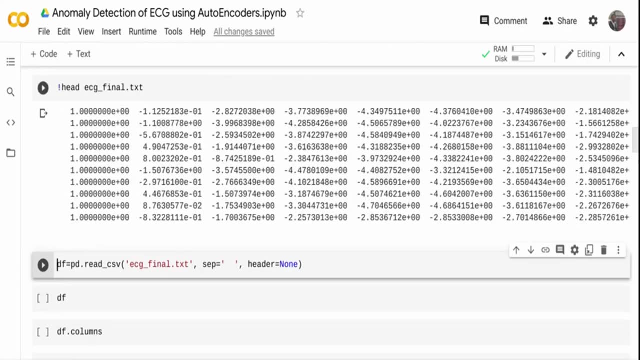 So I'm running this cat and then I'm printing the top few records of the file, So you can see. this is how it looks like. There are around 140 observations, and this first variable is the target variable. It says whether the activity is normal or irregular. 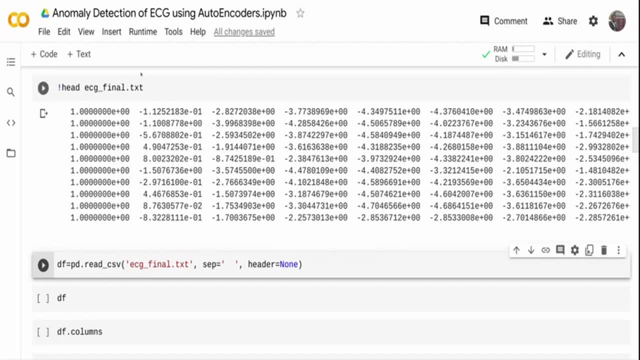 So let me first get it to the pandas data frame. So what I'm doing is I'm taking this particular ECG finaltxt, I am doing a read CSV. The separator is now a set of consecutive spaces, So I'm giving that as a separator and then I'm giving the header is not there. 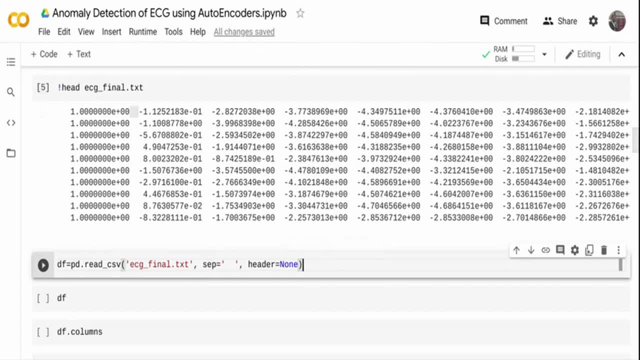 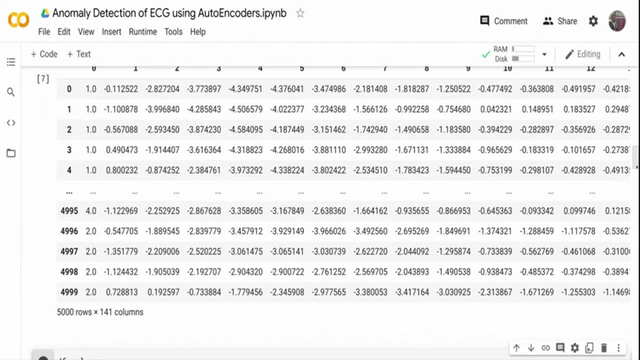 So header is none. If I don't give it, it will take the first line as header, So I'm taking that. So this is how my output looks like Now you can see like basically I have around 5,000 rows and 141 columns. 140 columns are 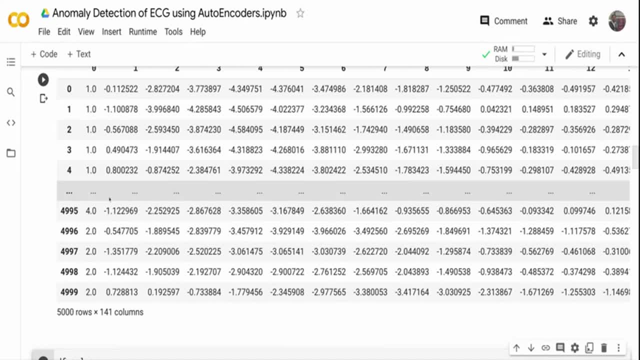 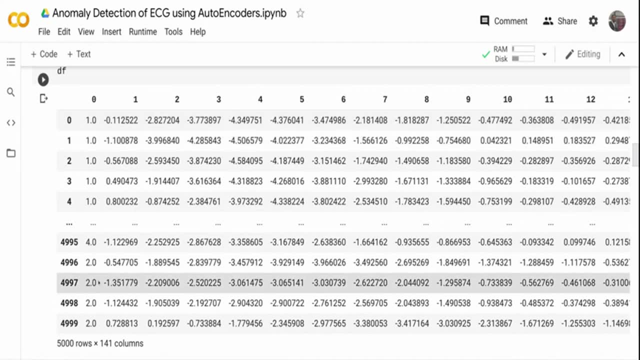 used to measure the art activity And one column is the target column. that is the first one. So now the class number one is the normal activity. The class number two, three, four and five are the irregular activity of the art. So that's how the output is. 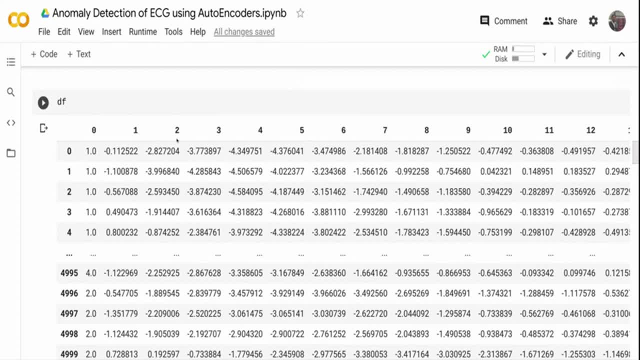 Now the column name, if you see on the top, starts with 0,, 1,, 2,, 3,, 4, that is a default column name that pandas give if you are not feeding any schema to it or if you are telling. 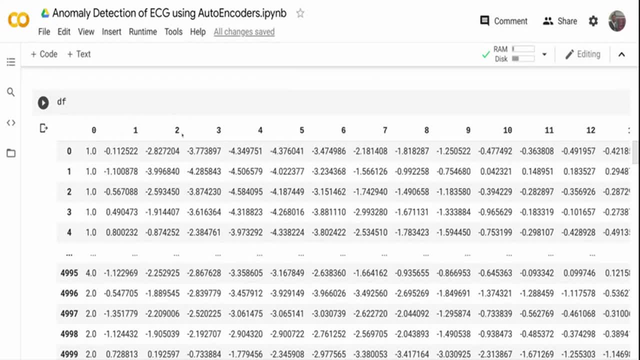 not to infer the header. Now, with this column name We cannot do any processing because the numeric in the column name- only numeric in the column name- pandas- does not allow to slice and dice right. So for that, what I'm doing is I'm just printing the column names. 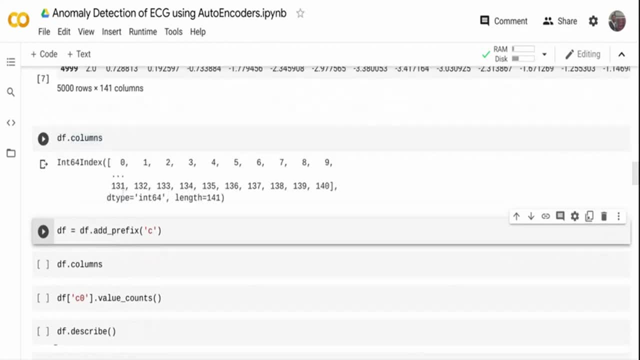 It starts from 0 to 141.. Now it says in data type I'm going to add a prefix to the column so that I can do some column processing And for that pandas has a function called add prefix. It can be had prefix or add suffix. 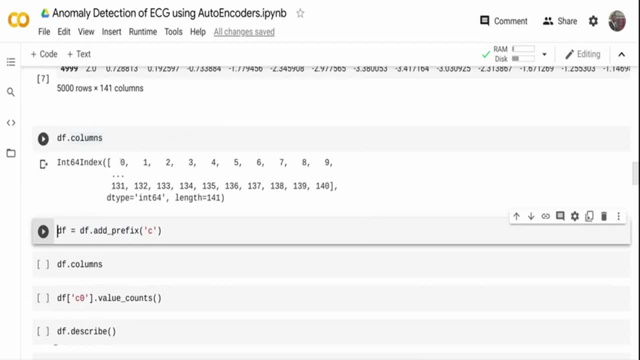 So I'm going to add prefix. So what will happen when I do this? The column name becomes C0, C1, C2,, C3, C4, so that I can slice and dice the column. Now, if you see the column name, the column name will be like: C0, C1, C2, C3, C4, right. 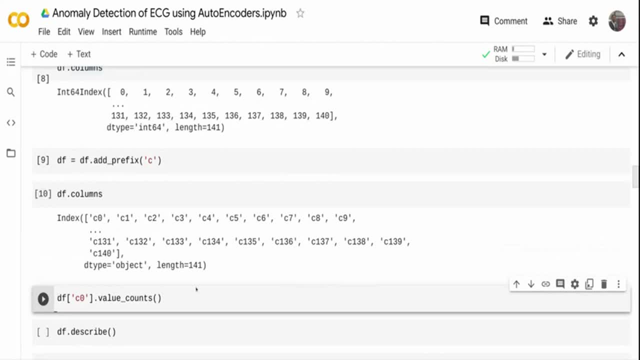 So now I can use this column name and then do a slice and dicing. Now, next, what I'm going to do is I'm currently focusing on the data preparation activity, right? So once we have the data preparation activity, we'll go to the modeling activity. 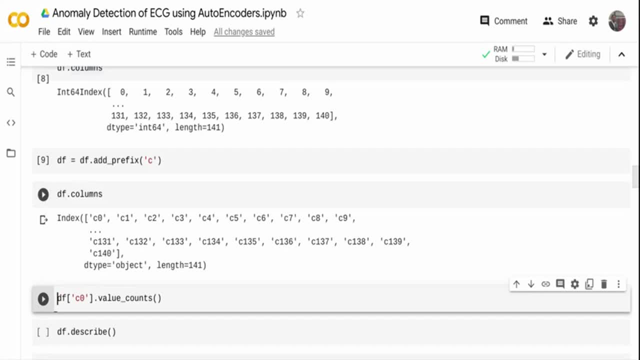 So now what I'm doing is C0 is my target value. I told you this is the first column. It tells It's a normal or abnormal art activity. So I'm just doing a value counts which will give me the number of records in each category. 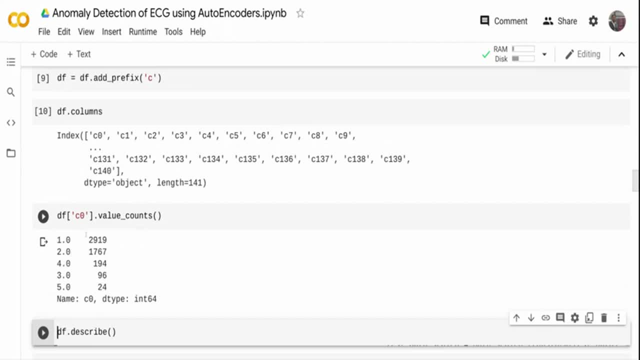 So, if you see, the data is between one to five and one has the most observation, that is, two, nine, one, nine, uh, the second to fifth are the abnormal activity. First is the normal activity And this is how the abnormal activity looks like: two, three, four, five. 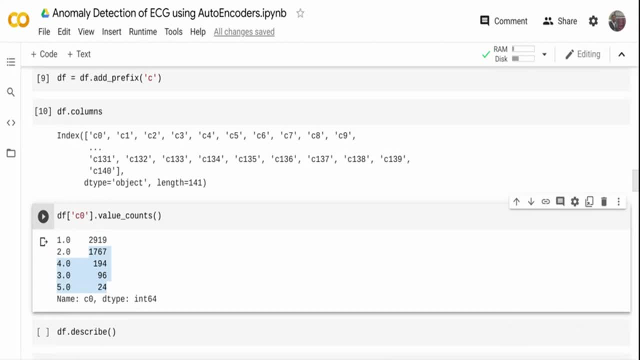 What I'm going to do is I'm going to combine two, three, four, five into anomaly and one into normal Right. That's what I'm going to do. So this is how the target distribution looks like, right. Let me quickly do and describe of the data set. 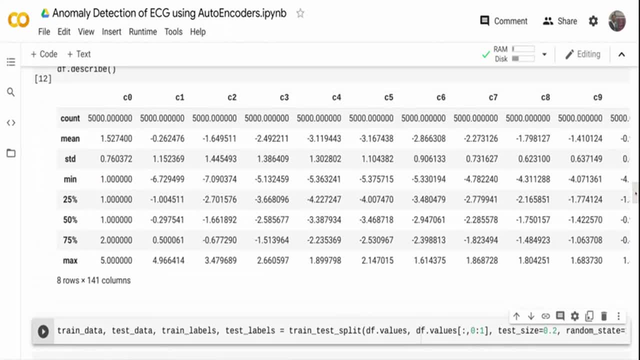 Uh, basically, uh, if you see like this how the data set looks like, this is how you are a distribution of data looks like of each column means standard deviation. Uh, if you see from the target column, the minimum value is one and the maximum value 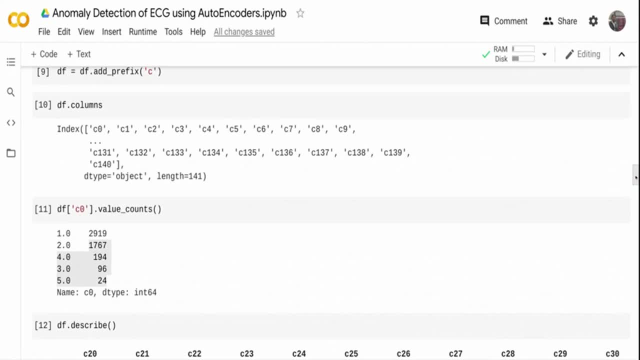 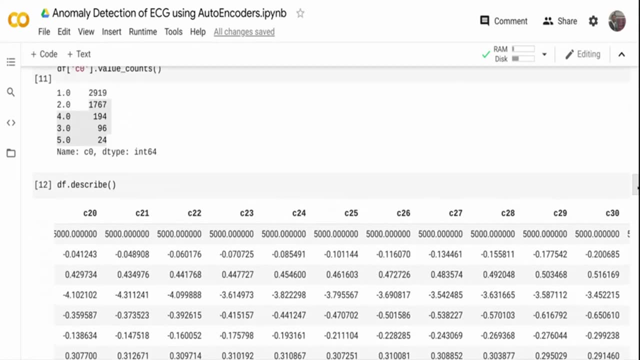 is five, Right. So this is how the data set looks like. Now what I'm going to do is I'm going to take this data. Okay, So I'm going to split the data set first, and for splitting the data set, I am using 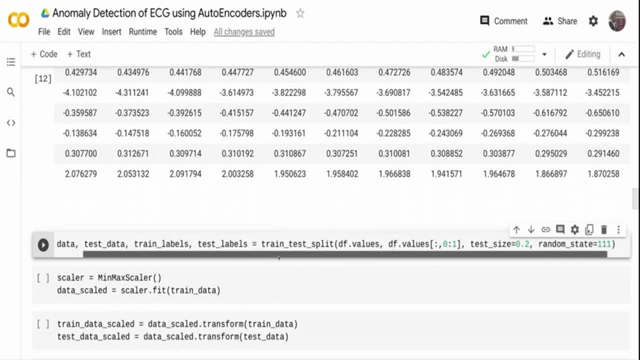 the train test split of a scikit-learn. I am passing basically all the values as my training, uh, from zero to one 41, and I'm taking only the first column as my target right. Basically, I need to pass X and Y value. 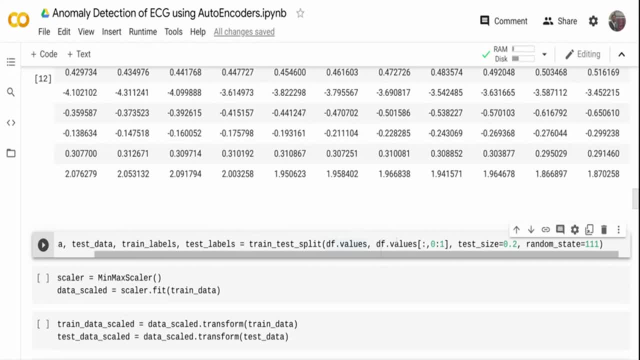 My X value is the feature columns. I'm passing all the data. My Y value is only the first column, uh, the C zero, which contains the actual um, which contains the actual label of the column right. And I'm telling you 80,, 20, split over here. 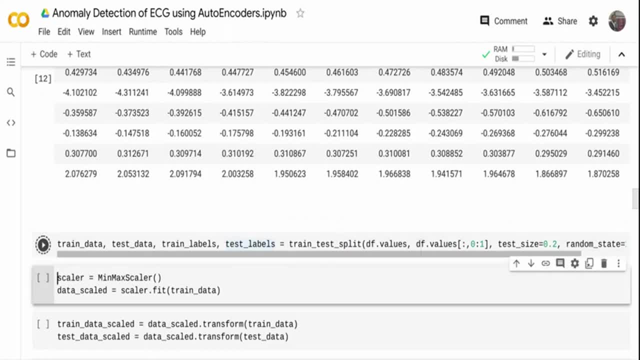 So once I run this, it will give me a train data and test data and train labels and test label, Right? So this is what it's given Basically for training. we don't need the first column because the first column is the label on the top. 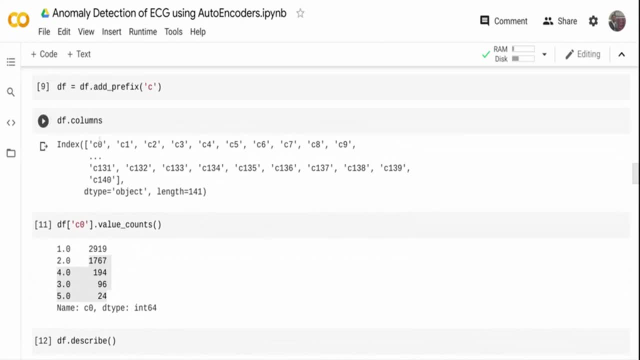 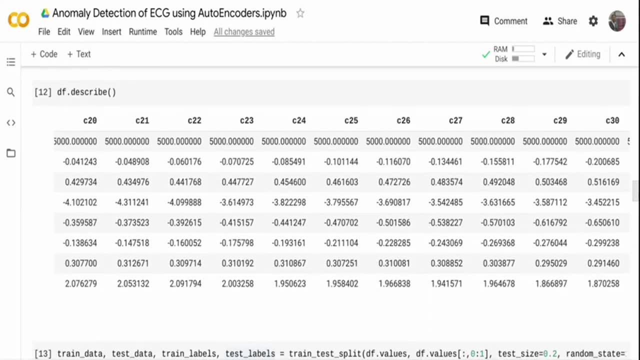 But the reason I kept it is so that I can split based on the columns uh, C, zero, uh, to normal and abnormal data set. That's why I kept it, but I will remove it. doing the training process right, Let's now go next. 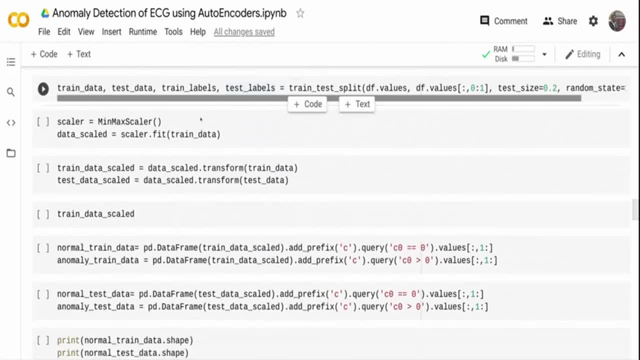 What I'm doing is I am basically, uh, initializing a scalar object now because I'm going to build a neural network model. Neural network model works better on a scale data right, It will train faster and it will converge faster. So I am doing a scaling. 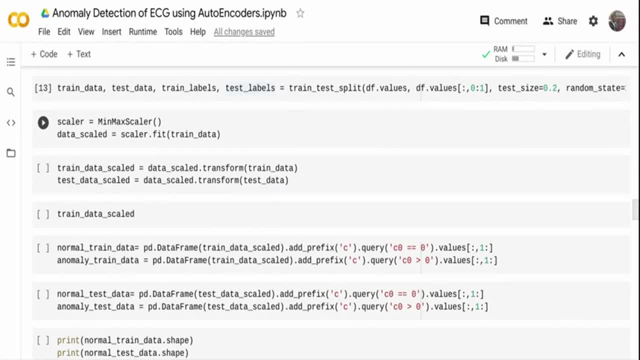 I am using a min-max scalar here, but you can also try with standard scalar, uh in this case. Uh, so I'm using a min-max scalar and what I'm going to do is I'm going to take the train data hello and scale the data right. 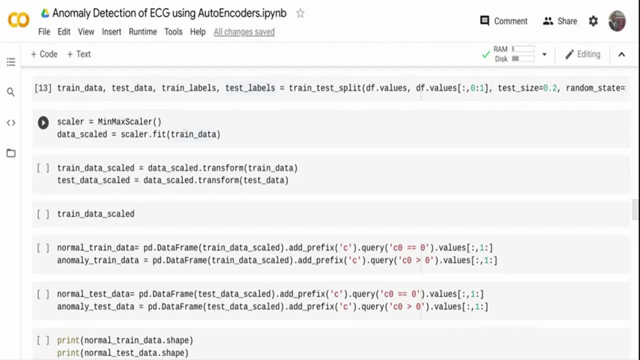 I'm going to basically uh fit the data set on the train data. Okay, So my my scalar function will learn the parameters using the train data and I'm going to use the learn parameter to transform the test data set. That's what I'm going to do. 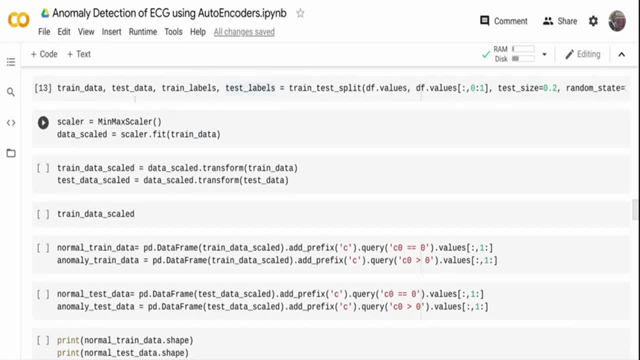 So I'm having a min-max scalar object initialized, I am calling scalar dot fit on train data And then I have the data scale, which is the learned parameters. Now what I'm doing is I am going to scale my training data and both test data. 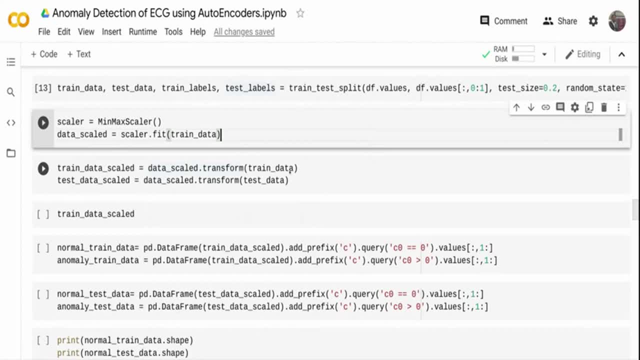 So I'm calling the transform function of uh transform function The train data and test data. So I'll have the scaled version of the train and test data set right. So now, if I uh run the output train data set scale, uh, basically it will have an complete 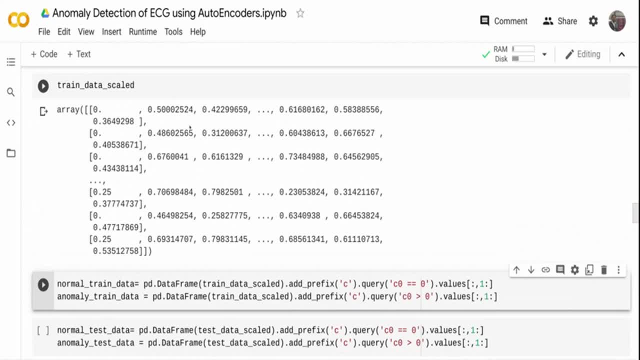 array of 141 values. Uh, this is how it basically looks like. even the input value is scaled, but that's fine, We are going to ignore the input value, right. So now I have the train data scale. right Now. what I'm going to do is I'm going to split this particular training data. 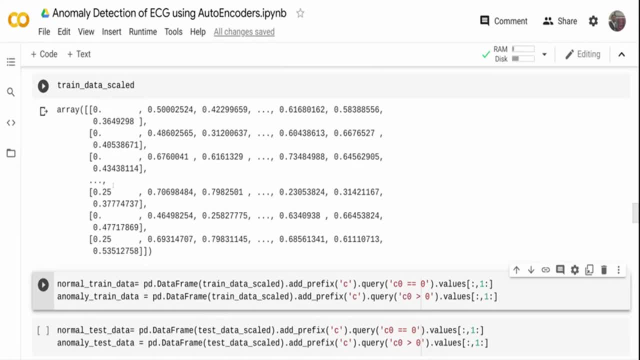 Okay, Into a normal data and anomaly data. And how do I know which is normal data and which is abnormal? data is basically based on the value train data scale. right, That's what it's going to be. I'm basically going to use: 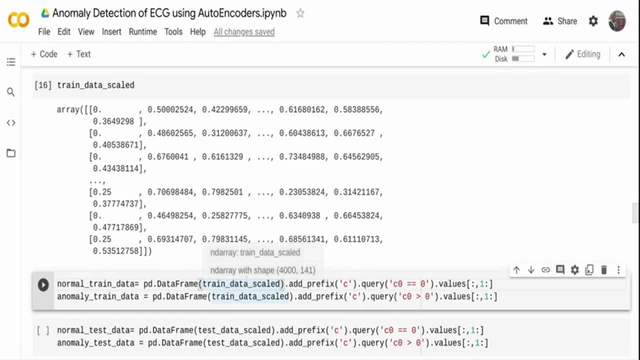 So what I'm doing in this case is basically I am taking the train underscore data scale right, And then I am uh, basically, like, um, uh, adding prefix to the column, because the column name, when I convert to Panda, it will be again zero: one, two, three, four. 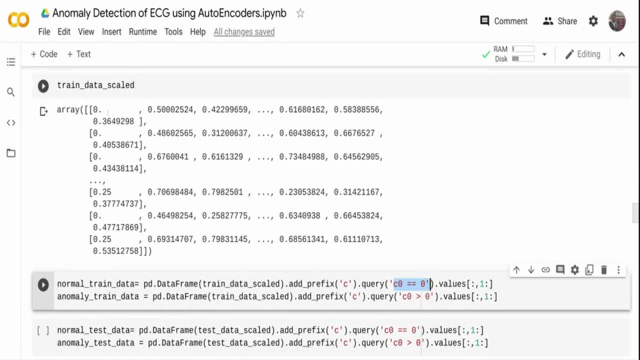 I'm telling: wherever the C zero, equal to zero over here, right? I'm basically telling: in this case it's it's a normal data, right. And then what I'm doing is I'm taking the anomaly data and I'm taking, again taking. 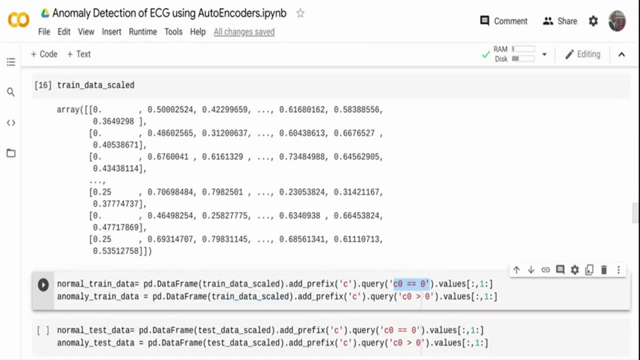 the train data scale and I'm querying based on the column greater than zero. Those are basically anomaly data for me. So I'm just uh taking that and I'm taking all the columns. that is after the first column, because first column is the label column. 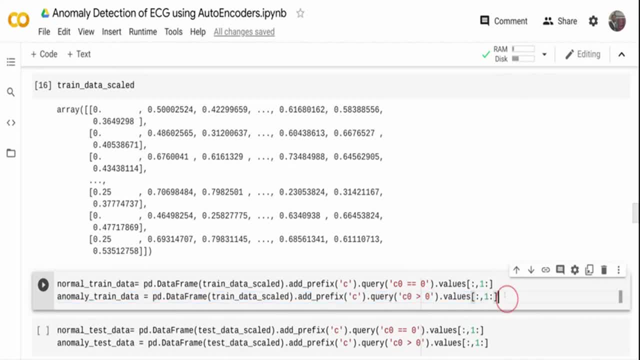 I'm taking all the data after the first column in this case. Okay, So it will give me a normal train data and anomaly train data. That's what it's going to do, So let me run this one, and now I have a normal anomaly data and train data. 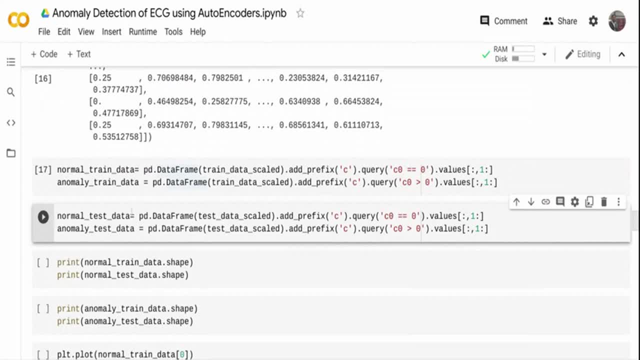 I'm going to do the same thing for test data as well. I am going to split into normal test data and anomaly test data, right? So let me run this part, So I will have, like normal uh test data and anomaly test data in this case, right? 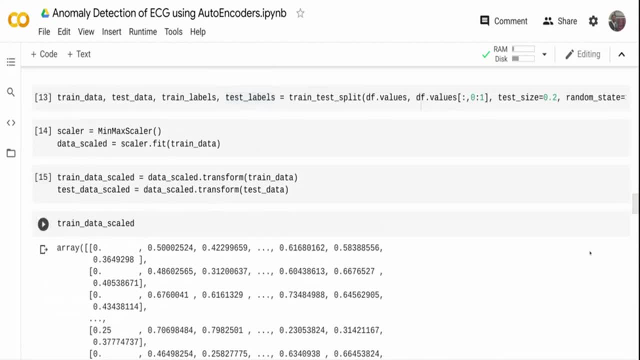 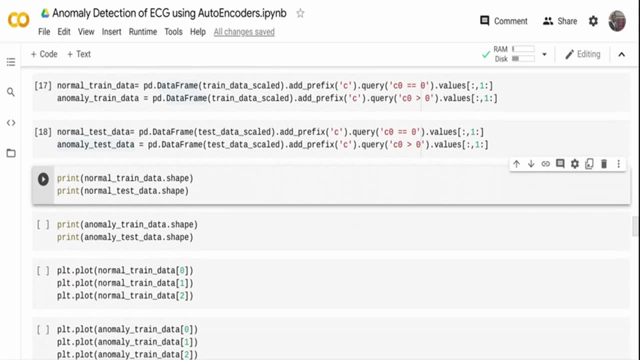 And here I am using the test data scaled over here which I'm using over here. Okay, So now I have a test data frame and a train data frame. Now the train data frame has its own anomaly and normal data set. The test data frame has its own normal and anomaly data set. right, 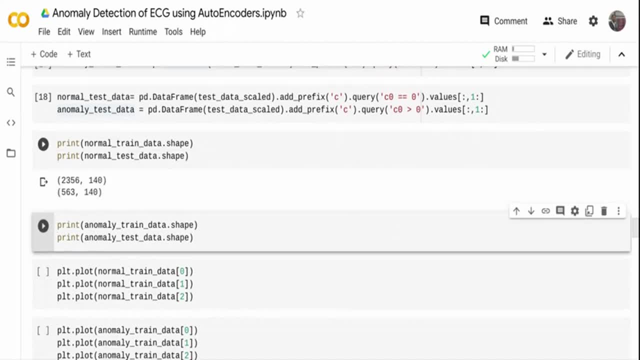 Let me quickly print the shape of it And this is how it looks. like it's 80, 20 split. You are two, two, three, five, six records for normal train data And uh for uh, normal test data. you have five, five, 63 records and similarly for anomaly. 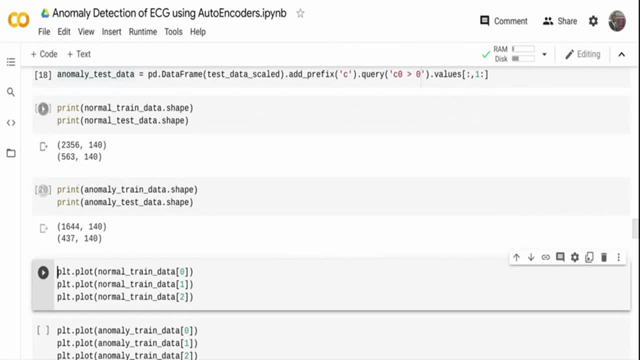 you have one, six, four, six records. You have one, two, three, four and four, 37. It's not like very highly imbalanced that we need to do anything. But anyway, like for auto encoder, we are going to train only with normal data set. 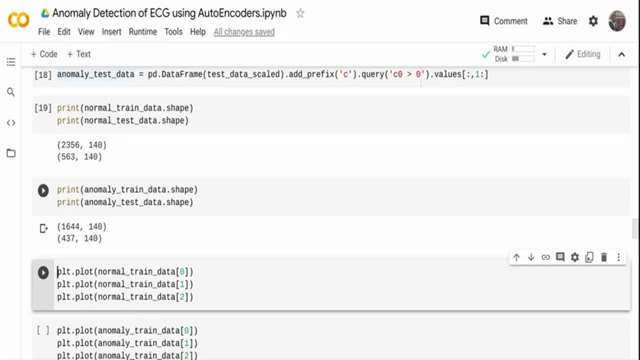 We are not going to use anomaly. Anomaly is going to use only doing the validation and inference, right? Uh, that I have covered in my previous video, but I will talk about that more Now. what I can do is I'm going to take some sample data- normal data- and plot it. 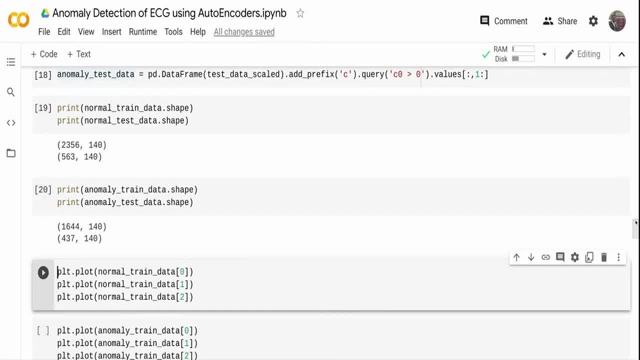 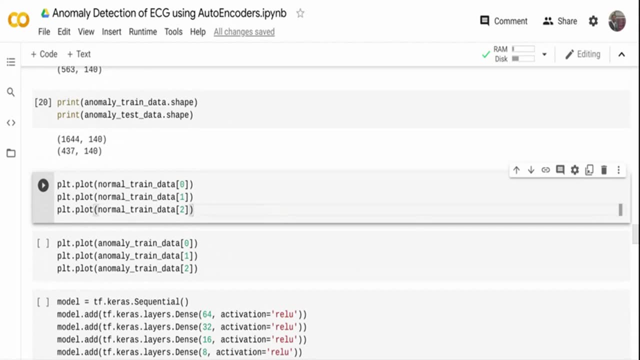 I'm going to take some of the anomaly data and plot it. I'm going to create plot can see how the data differs. right now, for auto encoder or for any anomaly detection, the data distribution has to be separate than your normal pattern, right? and that's what we are going to do. and we all know like auto encoder is an 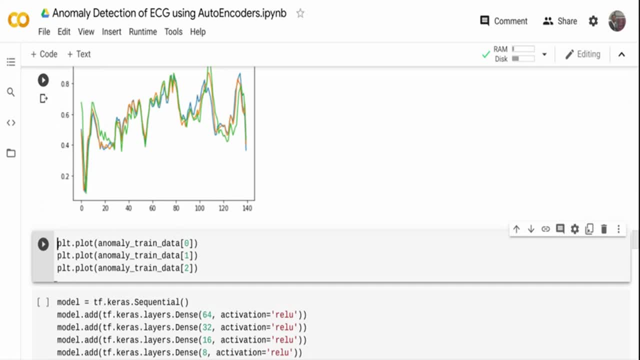 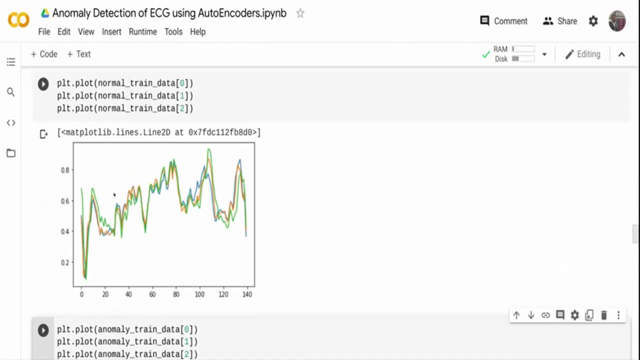 unsupervised learning technique so we are not going to feed labeled as target to for the model to learn. it's going to learn based on the pattern. right now, if you see this is the normal data pattern. I have the first three records plotted and if you see basically the activity, typically this is like 0 to 140. 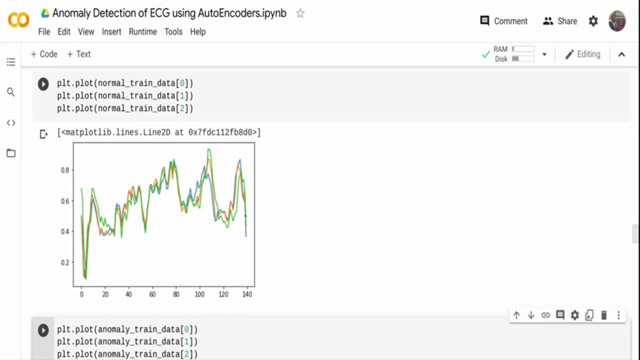 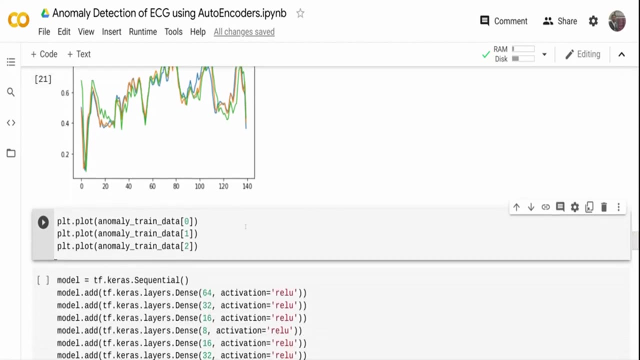 observations. the activity is trigger. basically there's up and down and this is how the normal pattern looks like. initially there's a drop because that is a start of the ECG measurement right. otherwise it's pretty much towards the normal cyclic circle right now if you take an anomaly data. in contrary, if you 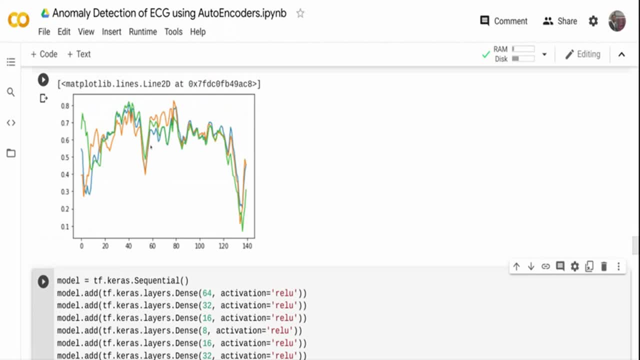 see basically now the anomaly data. it starts off to be normal, but certain there's a sudden drop towards the last observation and you can really see that the data is dropping. and you can see that the data is dropping. so we let's like that is a separation between the normal and anomaly in this case. right, so the what we are. 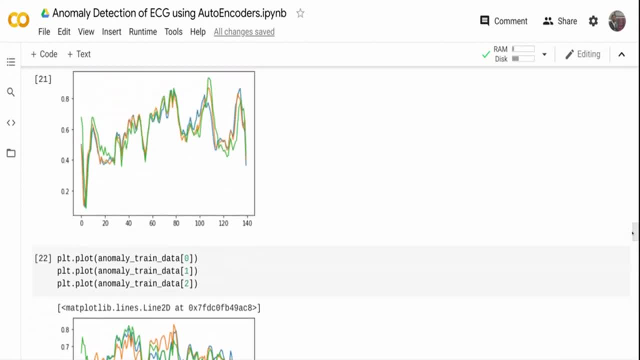 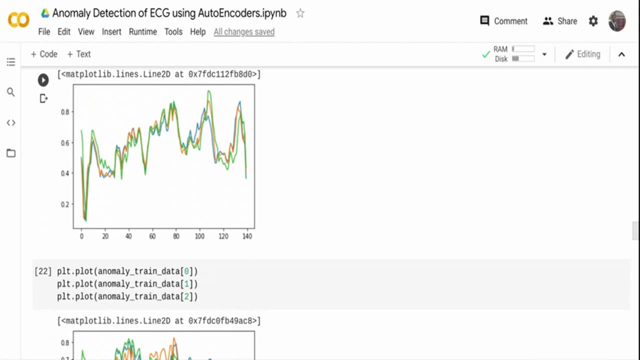 going to do in our model is basically take all the normal data observation. we will train a model that learns the normal data right and then we are going to use the anomaly during the inference process to see, like, how anomaly is. and if you remember, that is the term i said called reconstruction. 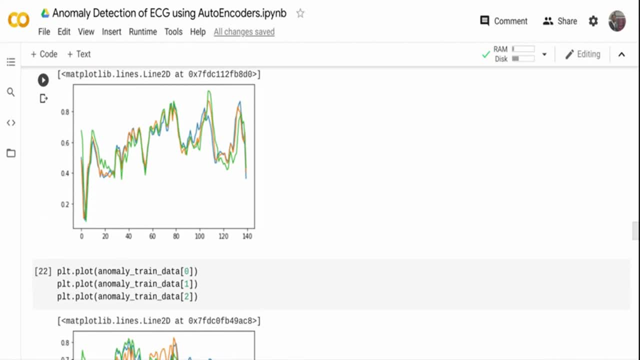 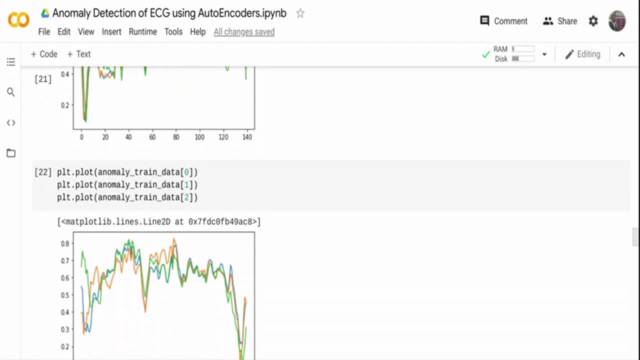 error. right, that's what we are going to use to determine whether it's anomaly data or a normal data. i will talk about it again. so the reconstruction error i had talked in my previous video, and that is, that is the basis for your anomaly detection- right, so now to create a model, a auto. 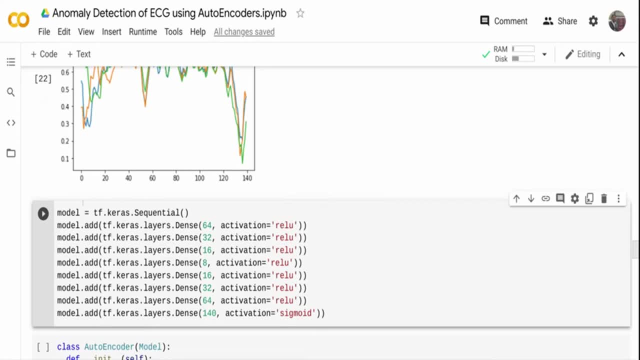 encoder. you have two ways to create it. one is you can just use the typical uh, the sequential model uh parameter that we have, and you can add layers in the layer. you are adding two layer, if you see. this is the encoder layer and this is the decoder layer. so auto encoder consists of basically an uh encoding part and 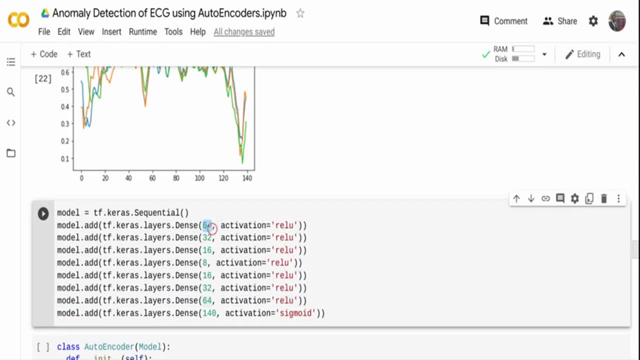 a decoding part. the encoding part, if you see, does it down sampling. it first has 64 units, 32 units, 60 to 16 units and it finally has an eight units, uh, intermediate layer. this intermediate layer is also called an bottleneck layer, so what it does is it takes a data in a 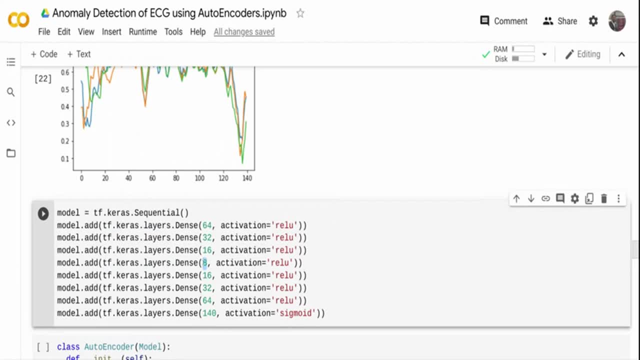 higher dimension and converts the data into a lower dimension, similar to a data compression. what a data compression does? so it has? it learns the embedding of the data into an uh eight unit vector- right in this case- and then to reconstruct back the data, it again uses an upsampler, which is 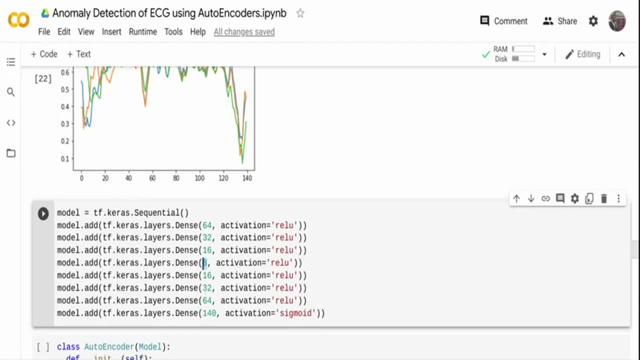 nothing but the inverse of the down sampler. so it takes 16, 30 to 64 and finally, the input for us is 140 units. the output also will be 140 units. now, in the process of taking this data, down sampling it and up sampling it, there is some reconstruction error. 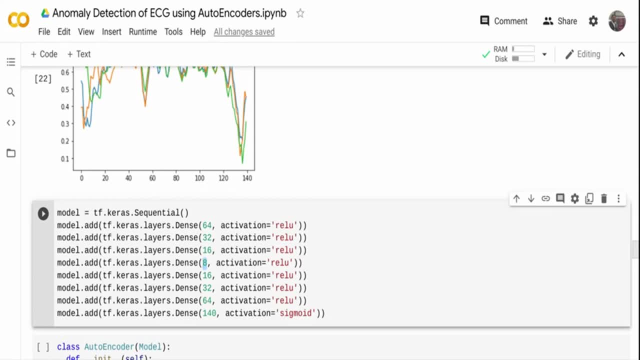 it's a lossy compression, so the data output will not be perfect right now. when we take a normal data and train this particular network, what is going to happen is it's going to kind of try to reconstruct the normal data, because that is our objective: to learn the normal data in a proper way. but when an irregular 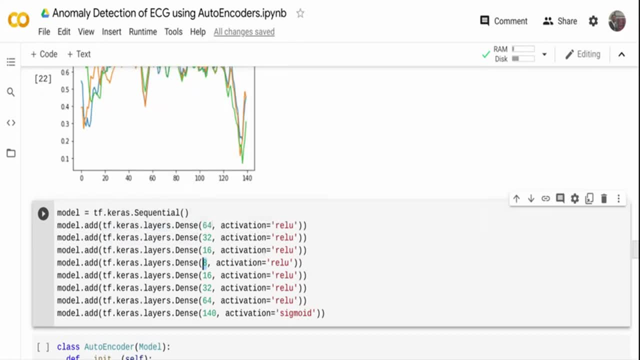 data- that is, the anomaly data- comes in, it will not be able to reconstruct at all. it will be completely the reconstruction error- the difference between the input and the output- is called the reconstruction error. the reconstruction error for the anomaly data will be very high compared to the normal data, and that's what. that's the thing we are going to use to determine whether the output 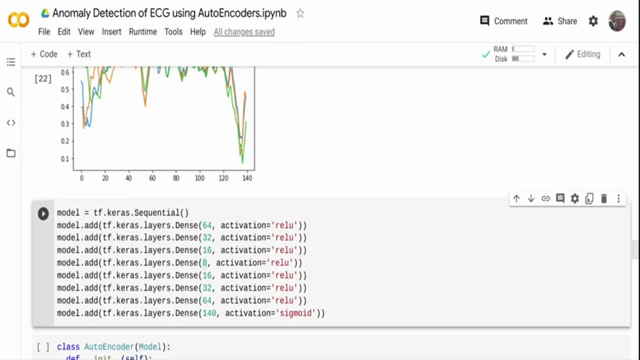 is anomaly or normal. right now, when we see the graphs and everything, we will get a better idea of what it looks like, even though it looks more theoretical now, where, once we go into the graph, you will be able to visualize it better. now there are two ways. you this one. 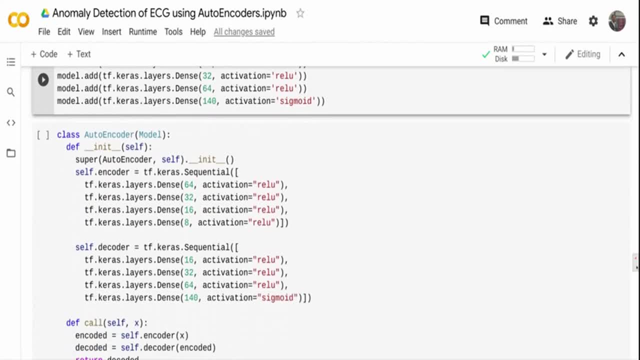 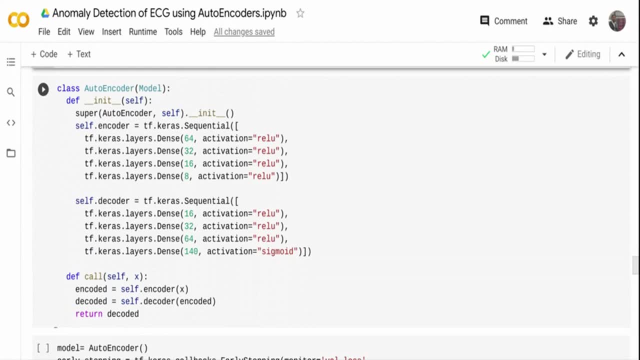 way of creating a model. the other way, uh, which we are going to use. this is subclassing right. the model subclassing parameter that is part of tensorflow 2.0 and why we use it is: it tells us to use the encoder and decoder separately easily, and in the top also. I. 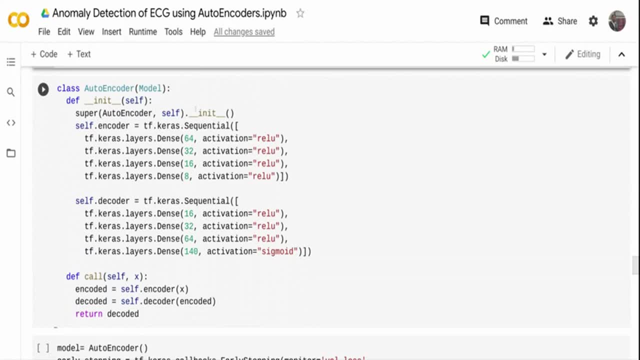 can use it. I can go to the layers and use it, but this gives you a better way of using the encoder and decoder. suppose I want to use this model only for compressing the data or for compressing the visualization, or take the output compression and run it. with this XGBoost or random forest model I can only use 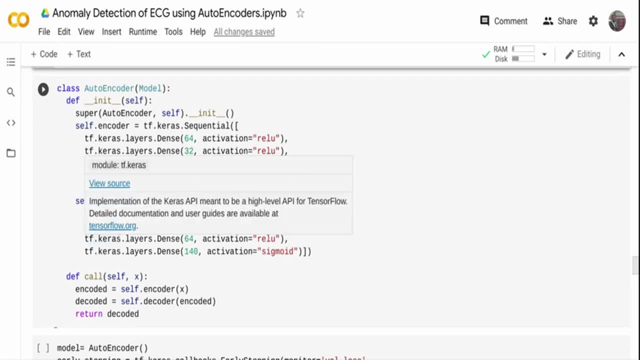 the encoder. I don't need the decoder at all, so this allows me to use the model in multiple different ways. so in this case, what I am doing is I'm creating a class autoencoder. right, I'm creating an unit function. this is the kind of a constructor that is getting called, and then what I am. 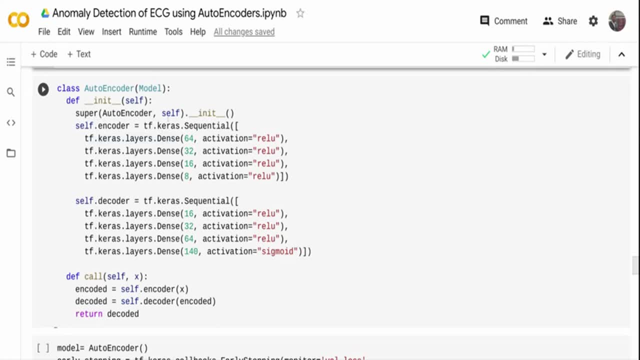 going to do is I am creating an encoder. the same thing in the sequential object that we create at 64, 32, 16 units and eight units is the bottleneck layer. and then I am having an decoder function that that's an up sampling of whatever the downsampling has been done by the encoder and finally the output is 140 units, in this case 140. 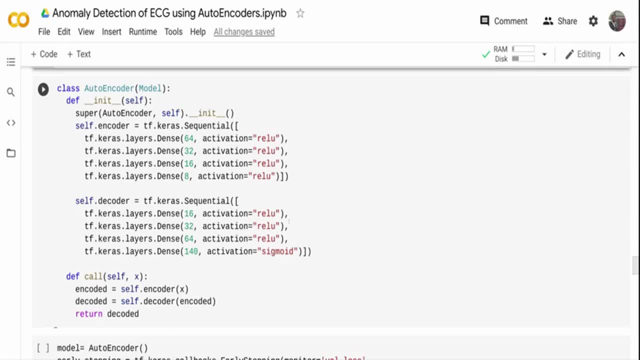 is the output. depending on your problem, you may want to change it. the final activation layer is sigmoid and remaining are a relu function. right, if you don't give, if you use an linear activation function, then your model is not going to learn the non-linearity. basically, you don't need this. 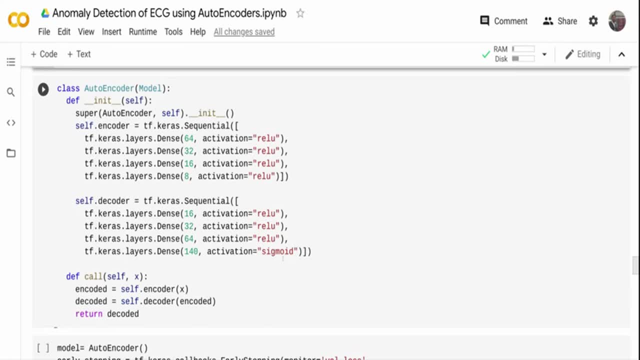 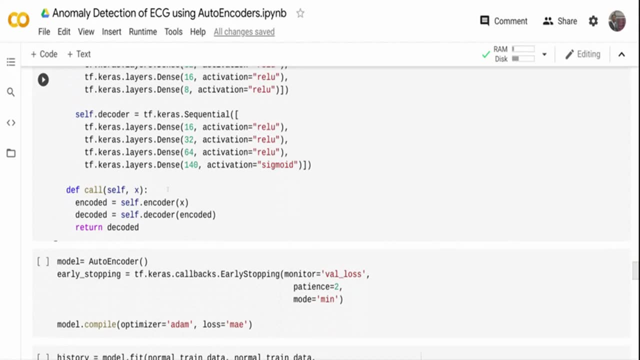 multiple layers at all, so i have non-linear activation, typically a sigmoid. i have, for the final output layer right now, the call method. what i am doing is i am basically calling the encoder, passing the input data and then basically i'm passing the encoder to the decoder and getting. 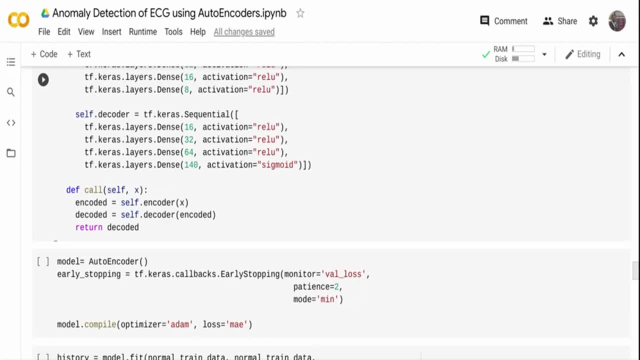 the output decoded value. so this is how my model looks like and let me run this now. this auto encoder is the class. once i call this class, it will return me a final model object. it will return me the decoded final model object which contains an encoder bottleneck layer. 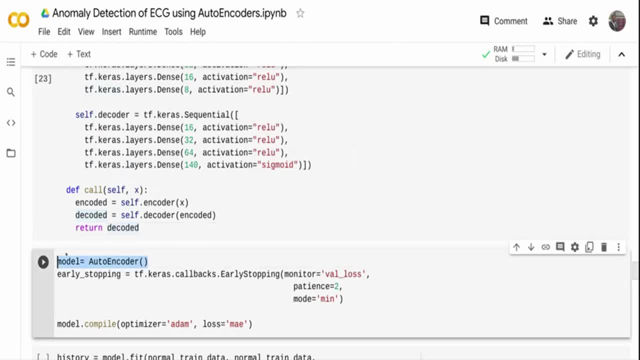 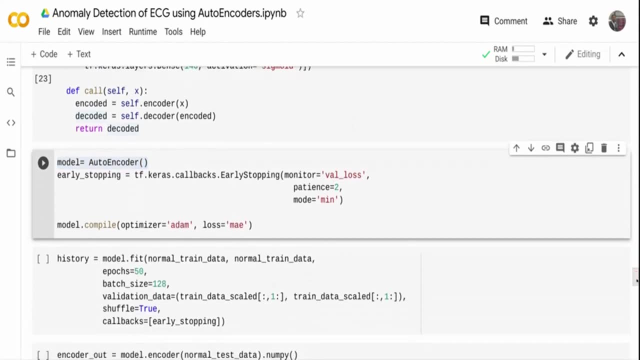 you and the decoder. that's what it's going to return. so i'm getting the model object by auto encoder. i am setting an early stopping function. uh, i want to stop my model in case the validation loss does not improve. uh, for more than uh two. two, two runs right, uh, two epochs. so that's why. 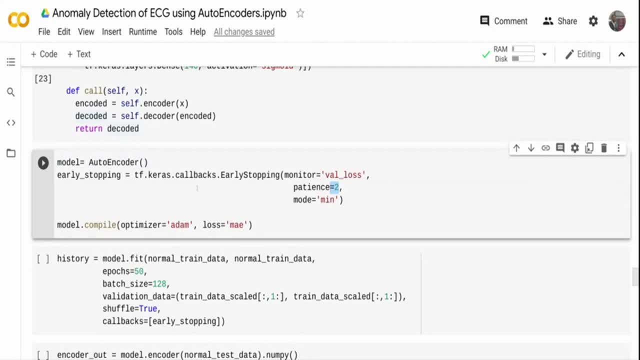 i'm setting the patient to two, patients to two, and then, uh, a mode is not required: validation loss: we always check the minimum. uh, if it's accuracy, we always check the maximum. uh, basically, if you don't set it, it will be auto, based on the objective that we are setting, the model we'll 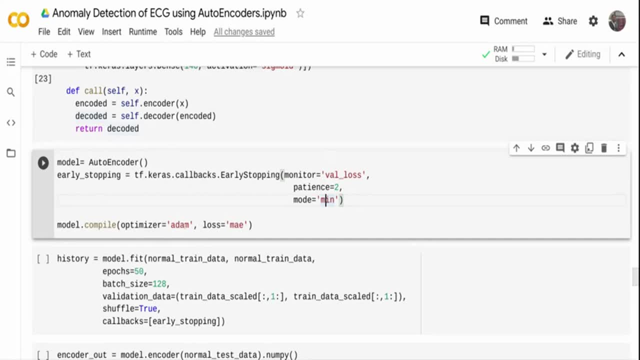 be able to understand. and then i'm compiling this model with an atom optimization- uh hand- and loss as a mean, absolute error. that's the loss function i'm going to use. so my model is defined. now i'm going to fit the model with the data. right now i have a normal data as my input and because it 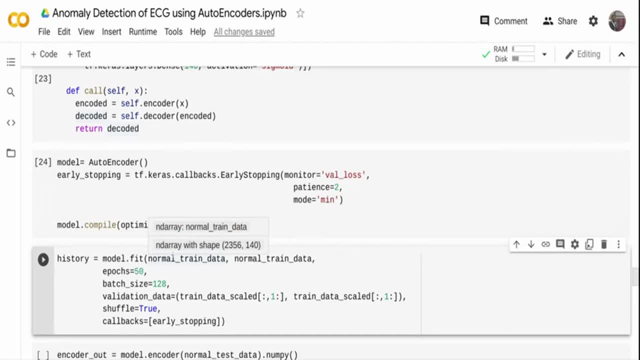 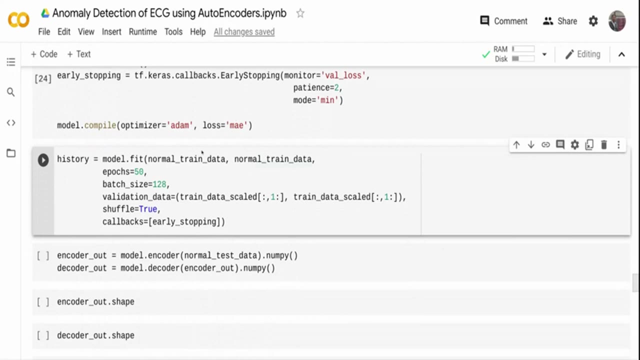 takes both s and y, x and y values and in this case, like uh, we see unsupervised learning. i'm just passing some dummy y values. that is, again i'm passing the train data, but because that's a mandatory field, otherwise you can just ignore this part. it's not going to get used now, if you see. 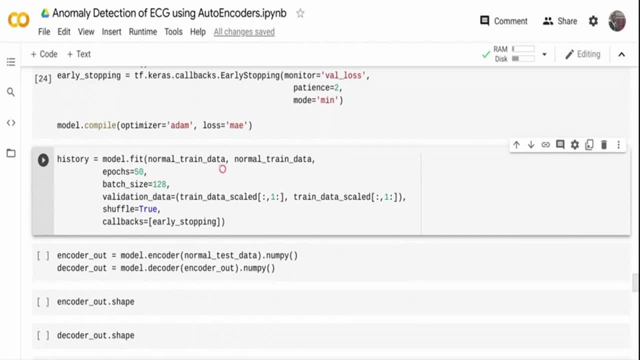 over here. what i'm doing is i am passing the normal data as input, so my model is going to learn the normal data, how the normal data looks like. it's going to kind of fit to the normal data right, and i'm telling my epochs as 50, but i have early stopping so it will not run for 50 epochs. i. 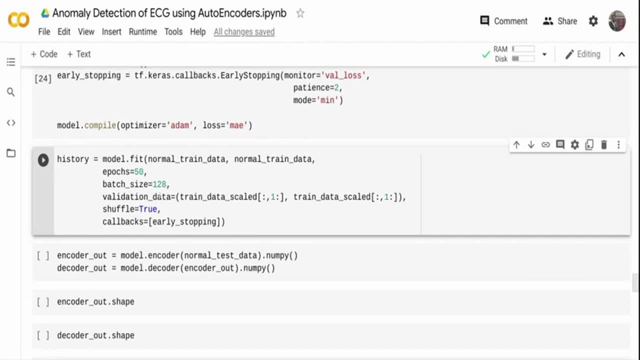 am giving a batch size and for validation, what i am doing is i am passing my entire data set, both- i'm not using the split data set- normally and anomaly. i am passing my actual train data that can contain that contains both the normal as well as the anomaly data. and why am i doing this? 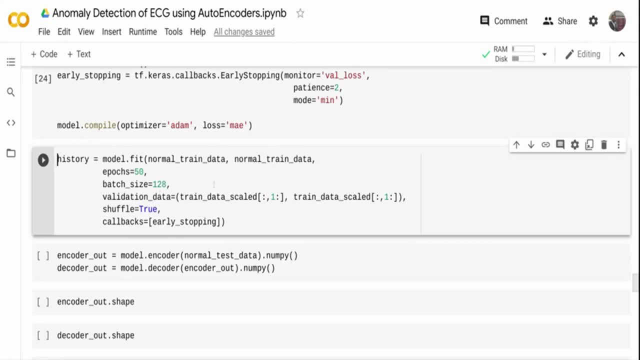 because when it's going to validate it it's going to basically go and do an uh comparison between the normal data and target data and wherever the normal data set is there, it's going to have a low, low, mean, absolute error. but for anomaly data it's trying to kind of fit to it but it will not find a. 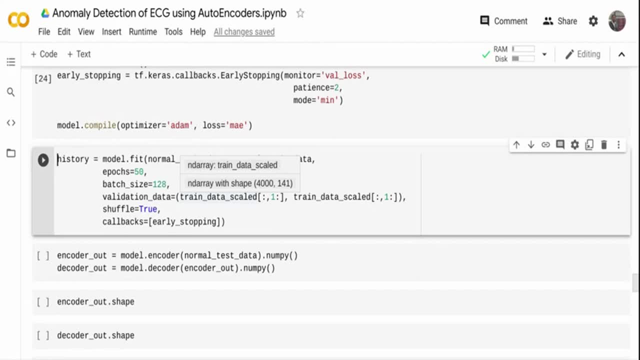 low mean absolute error. so it will try to separate the classes as well. right, that's the reason i am passing both the data set. i'm telling like, uh, shuffle equal to true. but if you are pass, if you see in the, in the case of time series data, the order is important, so you may shuffle equal to. 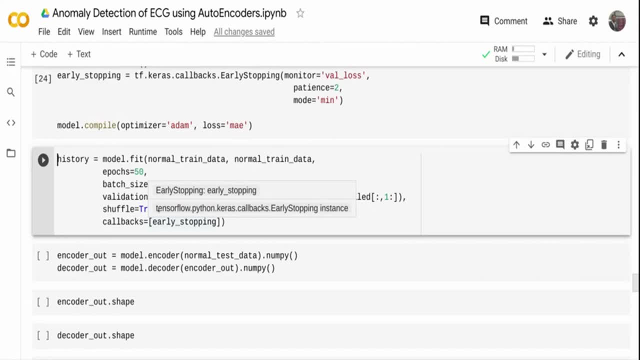 false and giving my uh callbacks early, stopping right. this is this. even though the ecg is a time series function right over the time, our art it is, but i'm not considering this as a time series function. if you are using an lstm model instead of a normal model and want to consider as time series, you may go for shuffle equal to false. 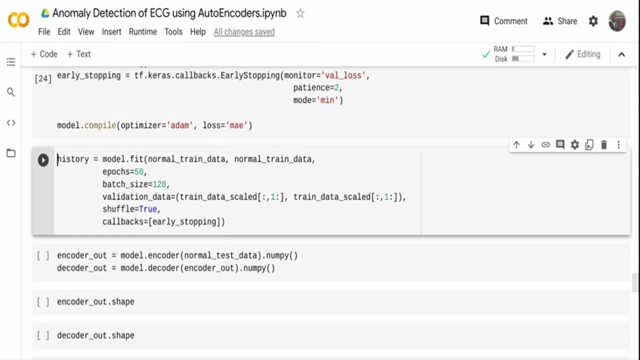 right, but in this case i'm just using a simple feed forward neural network. all right, so i have the early, early stopping callback. now let me try to fit the model. okay, so this will be very fast. uh, the unarmated one. so it's trying to run everything and you. one thing you may notice: 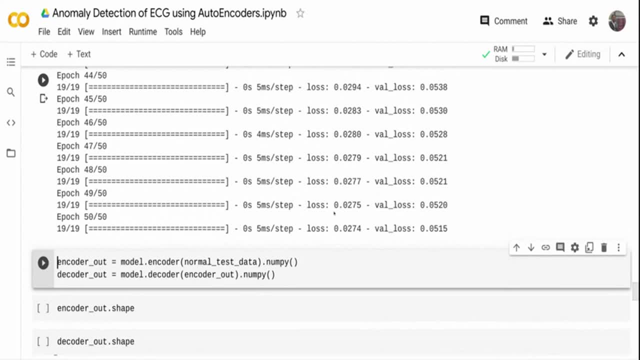 is the, the validation loss, and basically you are, uh, you are basically, uh, the normal loss, right, the training loss. there will be huge difference. so it's not that the model is under fitting in this case the reason. if you remember, in the validation function i am giving both the normal data and the 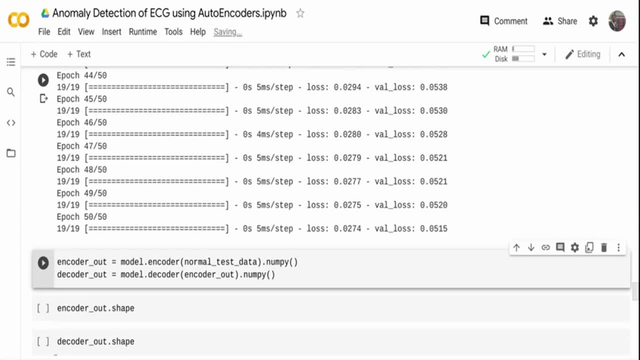 abnormal data against my training data as only normal data, so you will see this kind of behavior and auto encoder. that is completely fine and that's why i'm having early stopping, so that i can just validate the validation loss right? so it's not that the model has under fit, because my 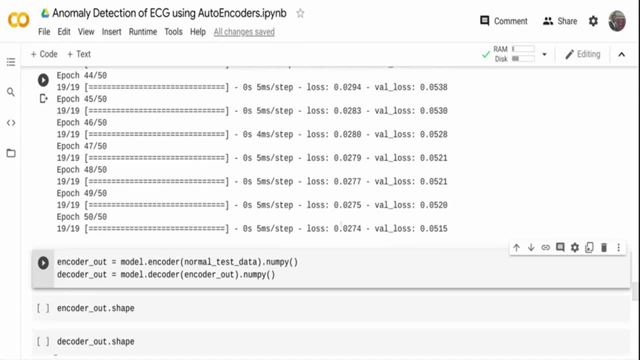 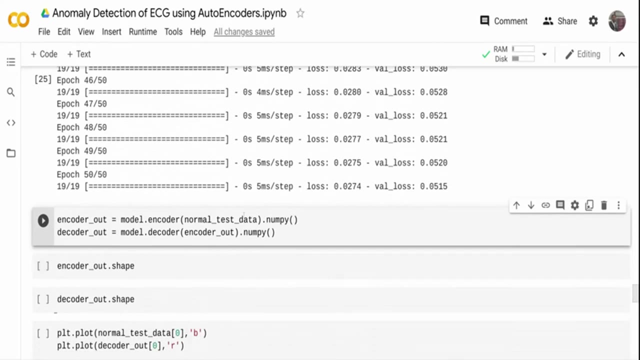 validation loss is way higher than my uh training loss. this is a normal behavior in auto encoder. okay now what i'm doing? my model is trained, i have a model, so now what i can do is i can get my encoder and decoder output separately and see like what it looks like- basically my encoder. 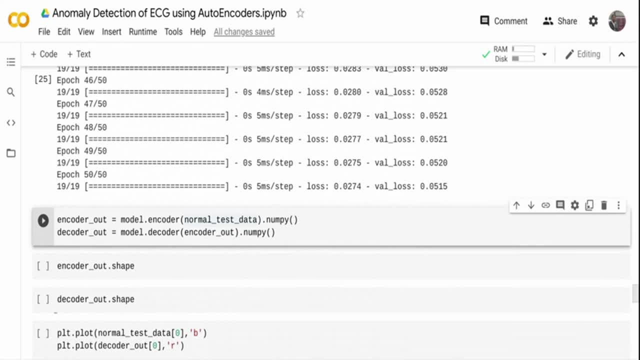 is nothing but a eight unit. uh, eight unit representation of the data. so i'm passing my input, which is the value of the data, and then i'm passing my input, which is the value of the data, my input, which is 140 units, and my encoder layer is a body as a bottleneck layer, which is eight. 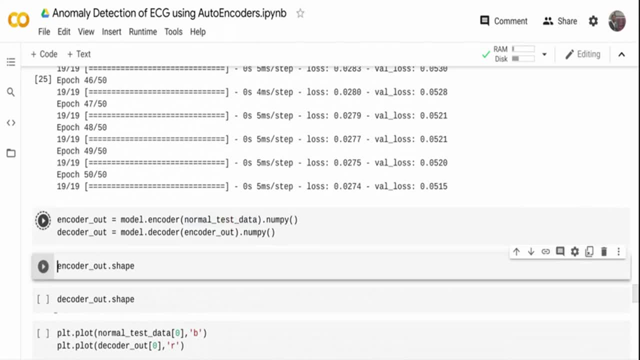 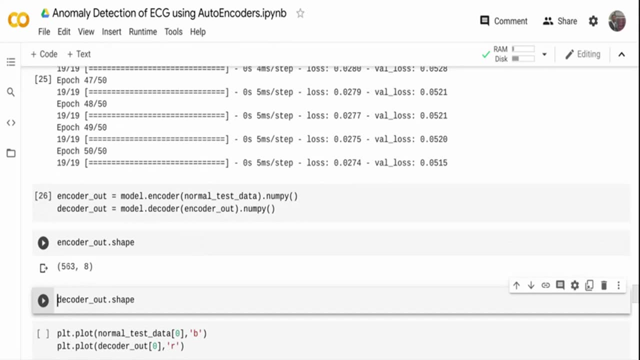 units. so let me run this and my decoder is constructing it back to one for 140 units. so if you see the output over here, my encoder output is basically like an eight unit uh vector and i am passing only the test data here, not the train data that was used during the training. 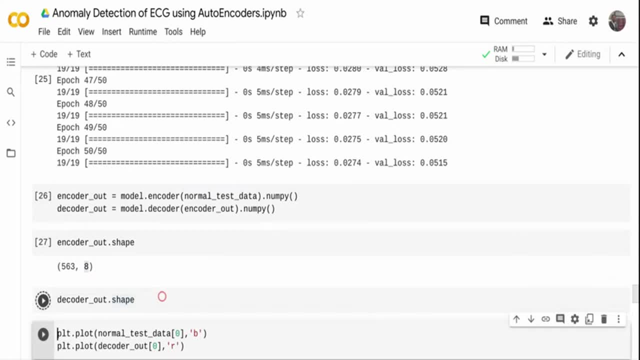 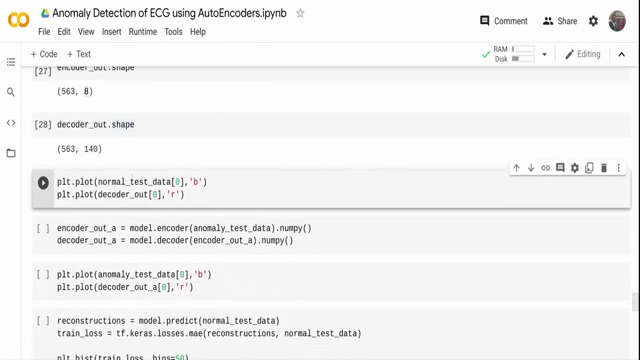 process and my decoder output will be like an 140 representation of the data, right, so this is how it looks like, so we can also quickly. what we can do is we can plot the normal data and the decoder output. the normal data is the actual data that we are fast passing. 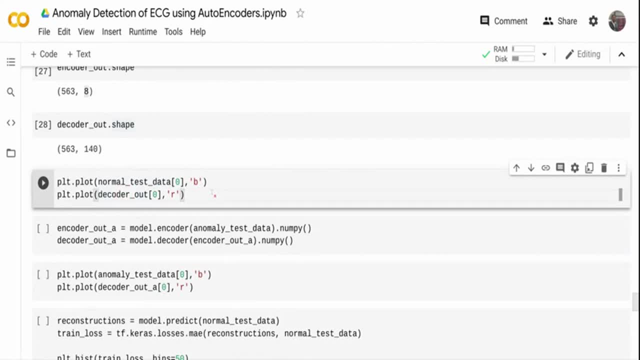 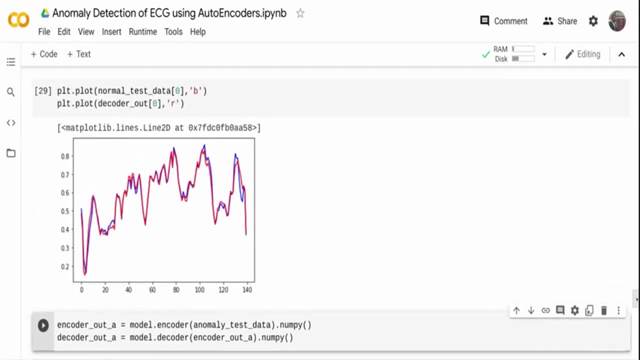 and the decoder data is the reconstructed data. now, what i said: the data will be similar, right, but it will not be exactly same. that may be some error. if you see this how it looks like, i have my normal data- that is the blue color, and i have my decoder data. that is the reconstructed data. 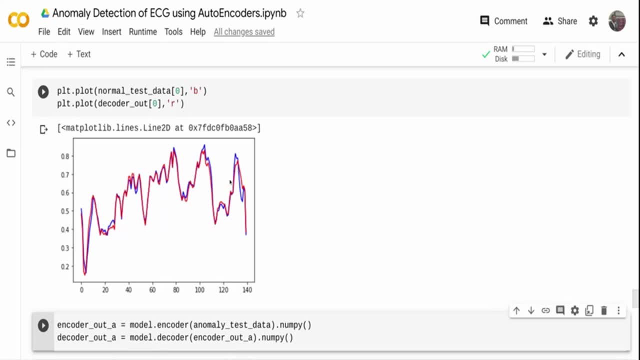 and if you see, there are some issues here here. here this is called the reconstruction error. the difference between your top peak and the red one, the blue and the red one, is called the reconstruction error and this is for normal data. if you see the normal data, it is fitting very well because our 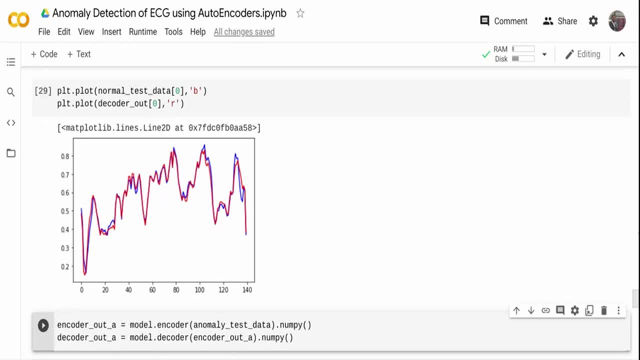 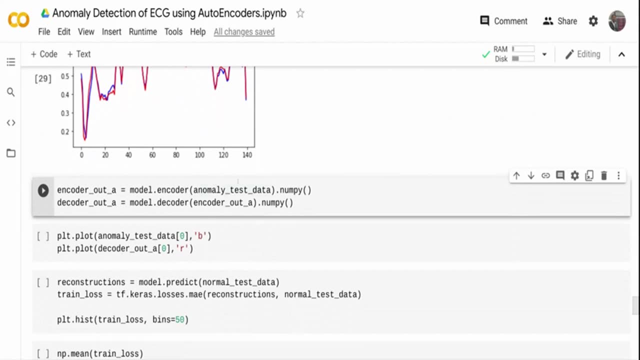 model was trained on normal data, but let's see what happens if we pass an anomaly data. so what i'm doing is i am basically in the. in case of the normal test data i passed on the top, i am passing on the decoder output. so now let me run this and let me plot how my anomaly test data looks like. 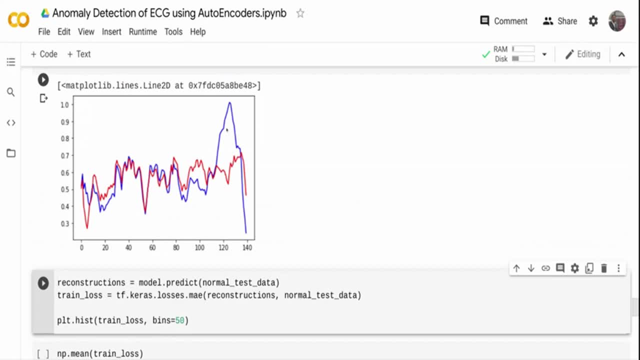 and the decoder output. now if you see over here the top one is my anomaly test data and the red one is my decoder output. if you see, basically here the error is pretty high, the reconstruction error in this case is pretty high and now basically we have got a pretty good model. 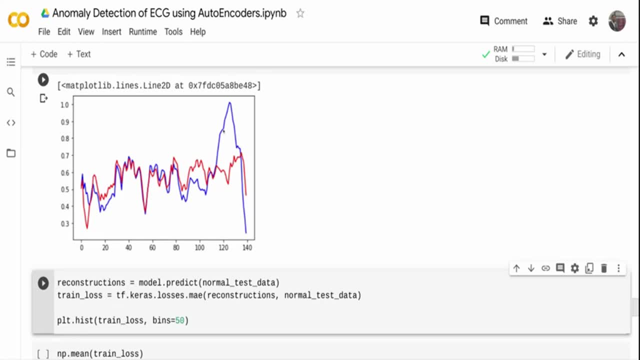 in case, if we pass an anomaly data, we are going to get i reconstruction error because it's not able to reconstruct the input over here. pass a normal data, it will, it knows about the normal data. so the reconstruction error is very less and this is what we are going to use in our case to basically see whether data is anomaly or. 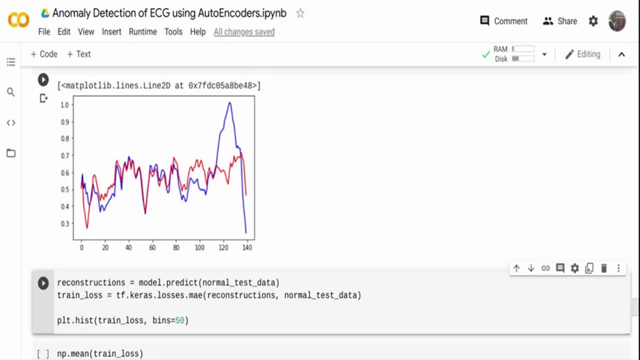 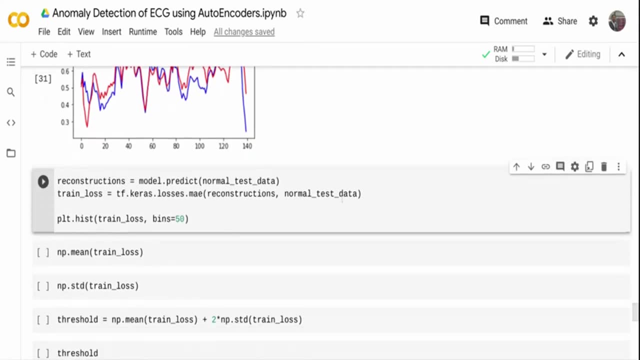 and data is, uh, basically a normal behavior, right? so now what we will do is we will define our loss like loss threshold for our model. so what i'm doing is i'm taking the normal test data, i'm taking my model and calling the model dot predict. so the it will. it will. 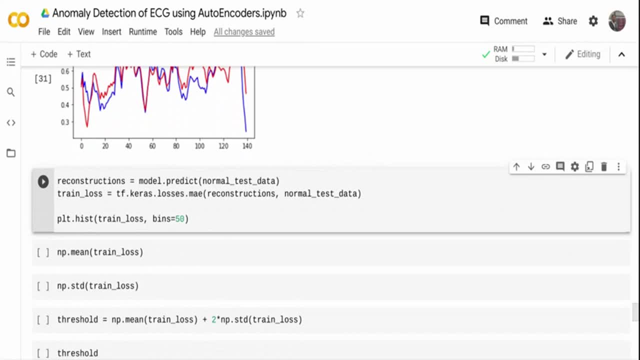 give me an output error between the input and output. right now what i'm doing is i am taking my uh- basically keras loss function on a mean absolute error. i am passing the reconstruction over here and the normal test data right, and i will get a loss between the normal data. 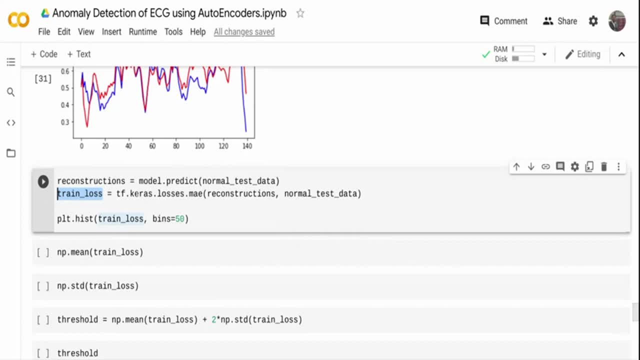 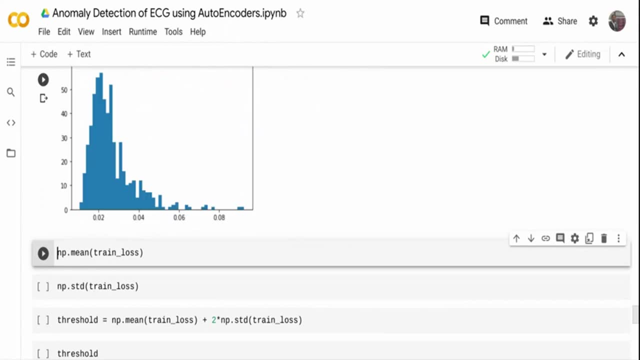 and your reconstructed data and i'm just going to plot it how it looks like, right? so let me run this. i'm just plotting the error component, okay here. so my, i have my normal data, i have my reconstructed data. i'm checking the error between the two, normal data and reconstructed data. 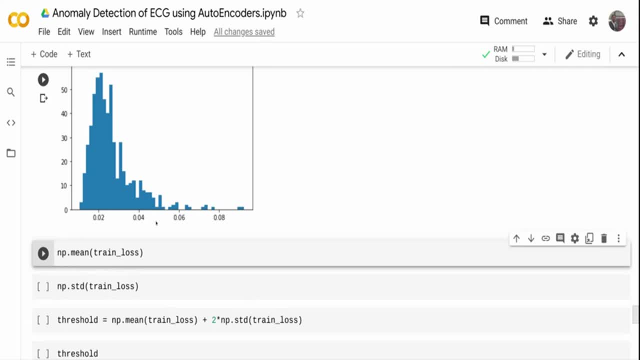 and this is how my error looks like. if you see the x-axis over here, most of my value lies between somewhere like 0.05. there are few anomalies. right, that's fine, because you cannot have a 100 perfect model, but i will. i will kind of tell you like how it looks for anomaly as well. so this is how my 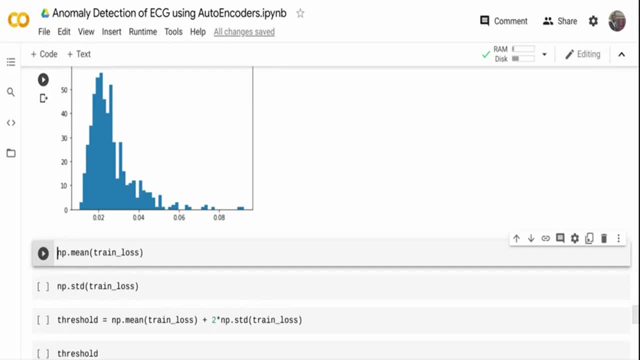 error looks like between my normal data and my reconstructed data. so typically it's around 0.05 of my observations are covered. right now. let me take mean of this train loss. so i need to set a threshold but from which i can tell any value above this is an anomaly or any value below this. 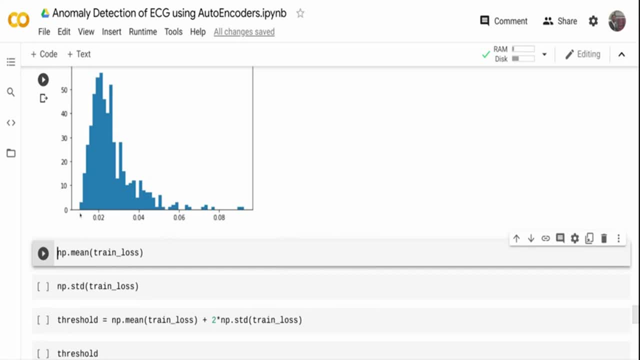 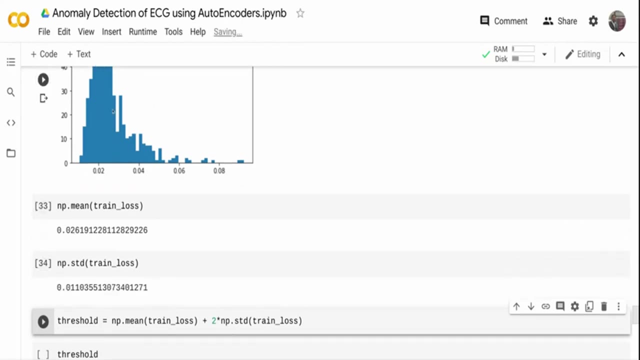 is a normal data right. so what i'm doing now, i'm going to take a mean of my particular uh training loss that i created for the normal data right. i am also taking the standard deviation over here. so for, in this case of the graph, 0.026, because most of the observation are in this range, 0.026 somewhere. here is going to be my mean. 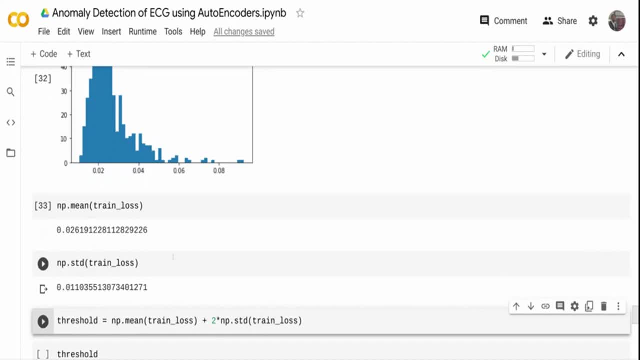 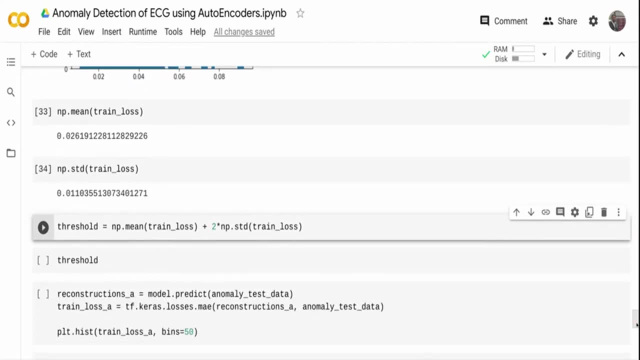 and my standard deviation is 0.01. now, to set a threshold, what i can do is based on the business scenario, the business context that you are dealing with. you can have one standard deviation, two standard deviation or three standard deviation, or four or five standard deviation as your threshold. 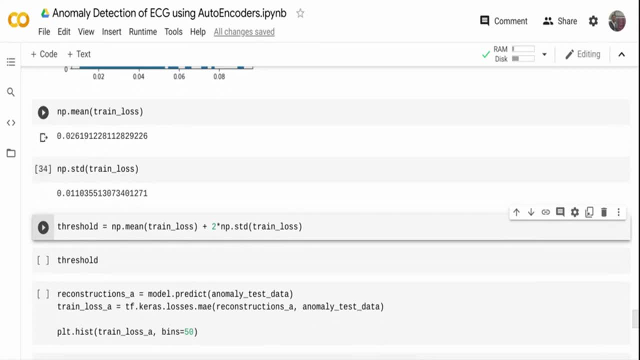 right, so i'm taking my threshold. i'm telling my, take my mean value, that is 0.026 and 0.001 is my threshold. so i'm taking the mean. i am having two standard deviation in this case, as my, as my total threshold, right, so i'm taking the mean. i am having two standard deviation of that mean. 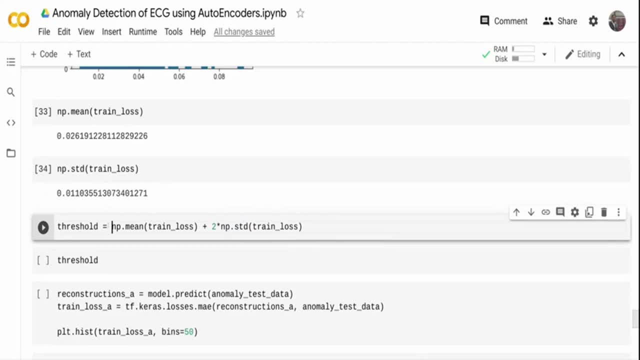 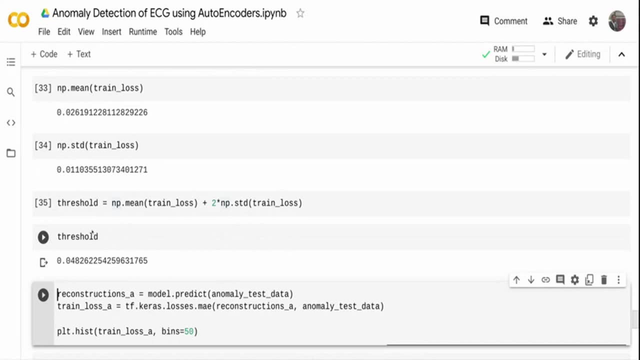 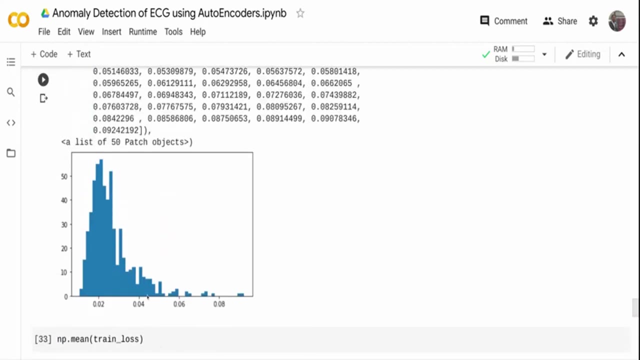 value of my standard deviation- uh value- and then i'm setting that as threshold. so once i run this, my threshold will be nothing but 0.026 plus 0.001 plus 0.001, right, so around 0.048 is my threshold. so my threshold above is somewhere here. 0.048 will be somewhere here. 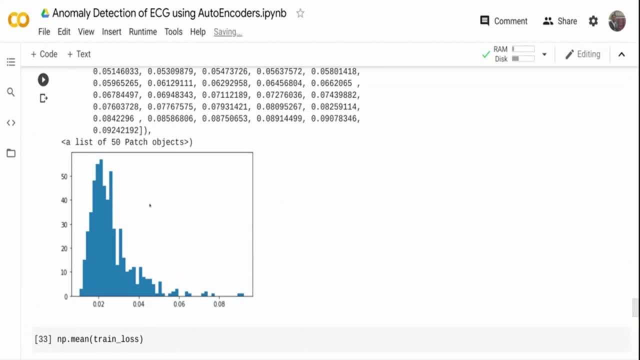 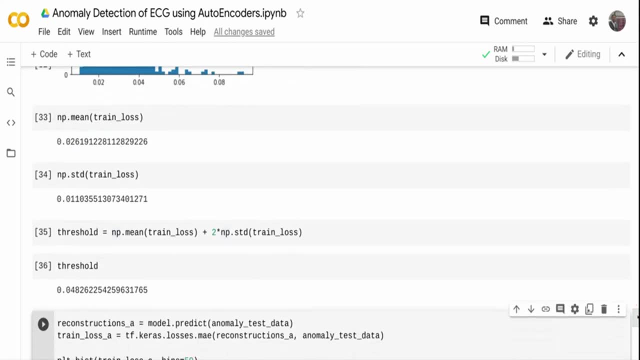 so this? so anything less than this threshold, because it's a normal data, the data is going to be normal. anything higher than the data, the normal is going to be abnormal or irregular. uh, pattern, right for us. now let me also do the same thing for the anomaly. 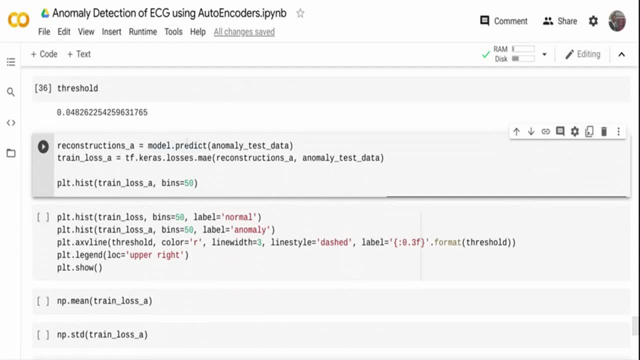 data right. what i am doing is i am doing my model dot predict over here. i'm telling like basically, uh, i'm paying the anomaly data and then i am doing the mean absolute error between the reconstruction a- this is the reconstruction anomaly and here the is thewny here. so that means as well as the stitch, so theues about. you put this closer to the single stress which you will be able to see. so that is a more easiest way of understanding the, the fitness of the data wizard. I want to explain what, how we keep this data and the data. 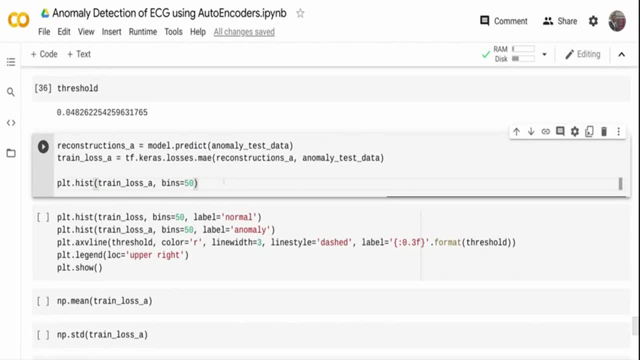 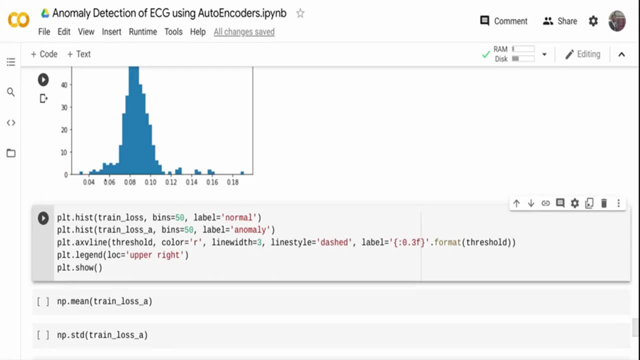 reconstruction anomaly with the anomaly test data and plotting the data right. if you saw on the top, most of our observations are within 0.05. but if you see over here, most of the for observation are hapu 0.045 or 0.05 in this case. so you can see the separation. if you see the x-axis on the top, 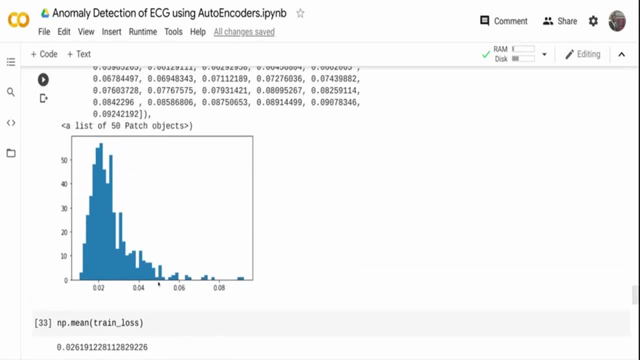 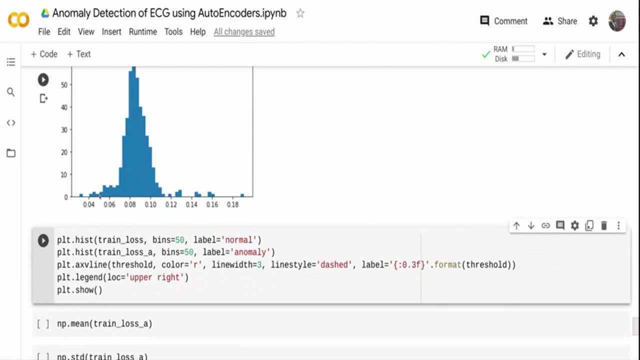 most of my data are within 0.05 range, all right, but here most of my data are above 0.05 range. so this says this shows my normal data and anomaly data error is completely separated. so i have a pretty good model, but let's plot both together so that we get a better idea of 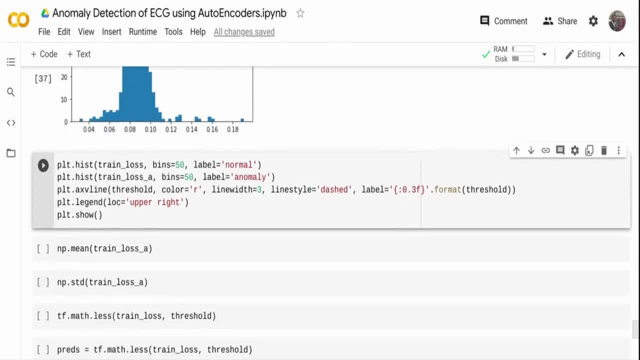 it looks like right. so what i'm doing is i'm passing my training loss, which is the normal training loss- this is an training loss which is my abnormal training loss, which is anomaly- and then i'm also plotting the threshold which i have set over here, which is nothing but this. 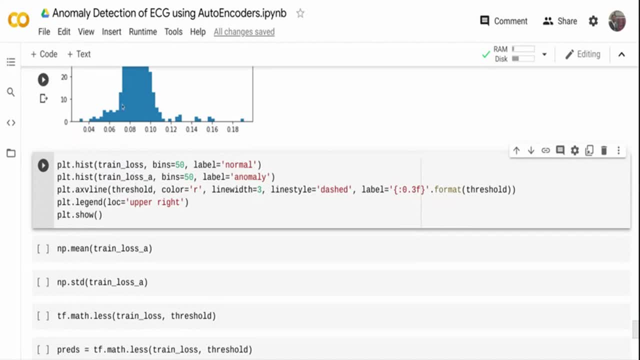 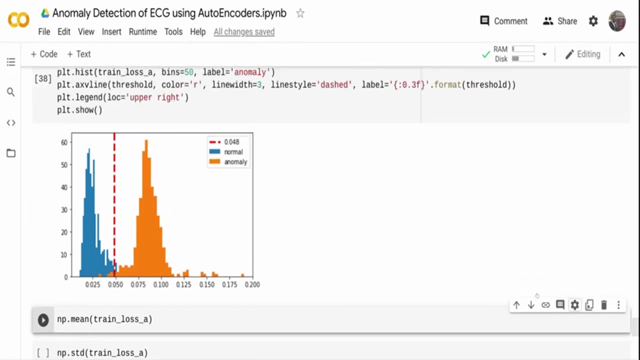 two standard deviation. so what i'm doing is i'm drawing a vertical, vertical line. this a x v line is a vertical line on the graph and i'm just plotting the legend. so this is how my output look likes. like, if you see on the left, the blue value over here is a normal data and the 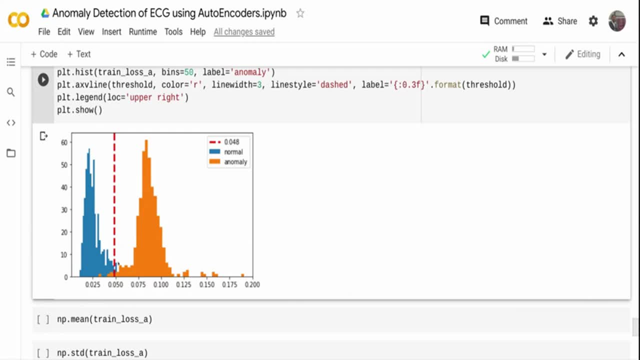 orange values are normally data and this is the threshold. if you see, over here i have few anomaly data in the blue region. so these are all going to be my false positives, right? uh, basically, i thought it's an anomaly, but it has detected. it's a normal behavior, but you can move. 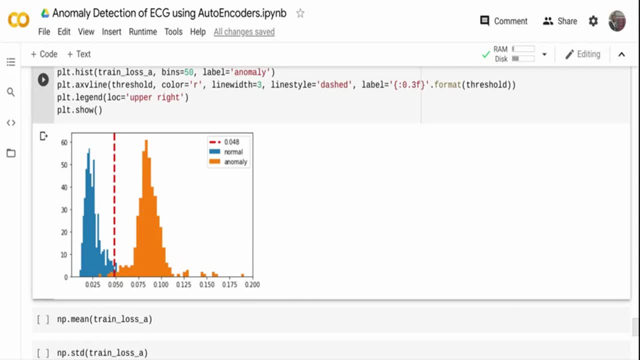 the threshold as per your business criteria. if you want to move one standard deviation, it will be able to detect more anomalies, but your purpose is to detect more normal behavior. then you can even make it three standard deviation of four standard deviation. it is all on your business scenario, right? my threshold is 0.048 right now. in this case, if 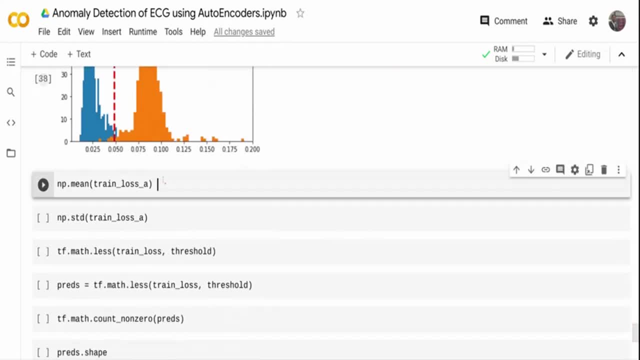 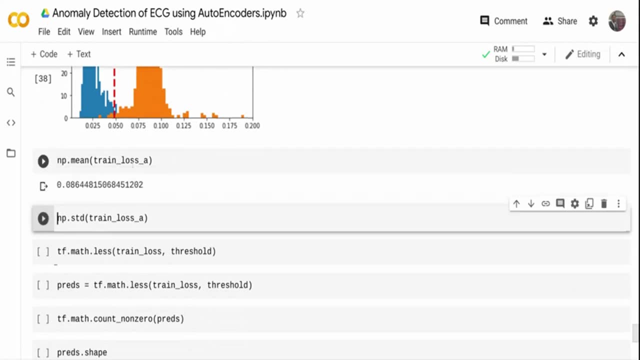 you see my uh me mean loss function for your anomaly data. you can see my mean earlier, the mean 0.026, but it's 0.86, way far apart. so so the mean is around here, 0.86 and the standard deviation is basically going to be uh close to the similar right because from the mean you are going to take. 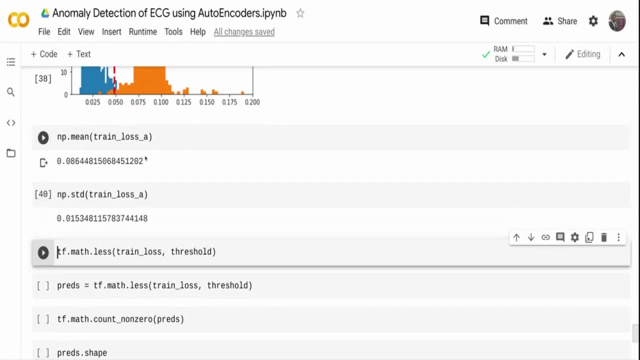 the standard deviation, right. so this is how it looks like. so we are able to build a anomaly detector using auto encoder which is able to very well separate your normal class and anomaly class, right, and that's what the auto encoder does. now let's see like how well our model has performed. 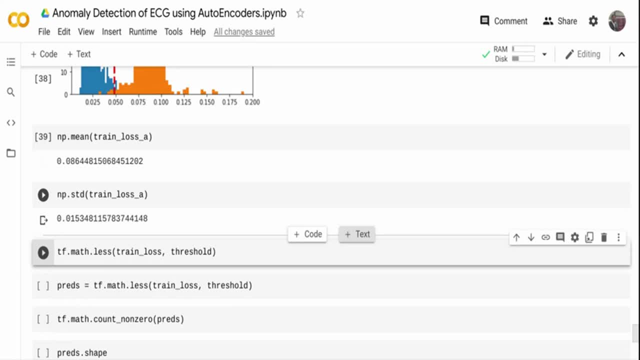 what is the false positives and what is the false negative. so what i'm going to do is first i'm going to find, uh, how well it predicted normal class right. so for that i'm using, like tensorflow math function, less i'm checking how many values in the training loss that we created for the normal data. 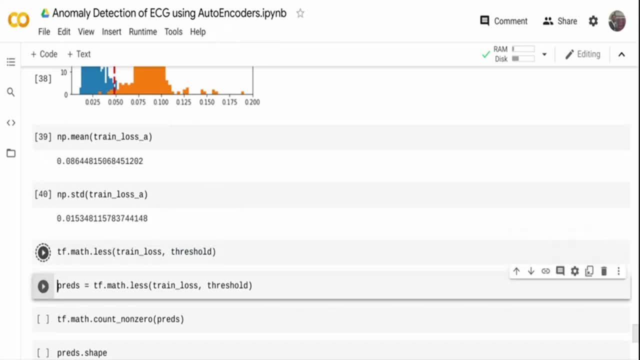 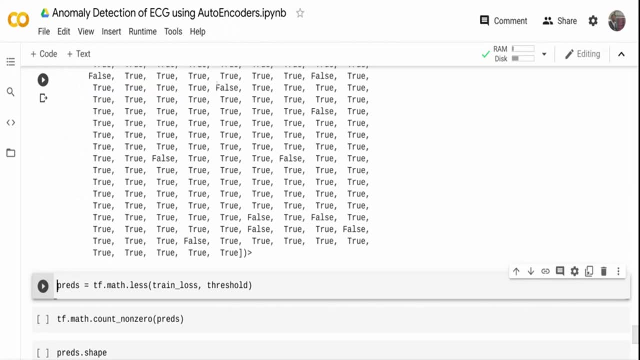 is less than the threshold right. so this will give me how many values are less than this. just i'm printing. it's going to: wherever it's going, it's less is going to tell true wherever it is more. so what i'm doing is i'm just passing that to an uh predicted object which will have nothing but. 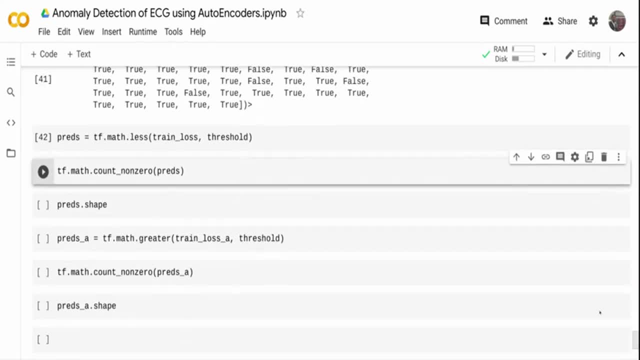 this array of true and false and then i'm counting non-zero. so what non-zero will tell? wherever it is true, it is non-zero by default, like boolean true is one and boolean false is zero. so i'm doing a math: uh, count zero and predicted it's going to tell how many. is it predicted correctly? because 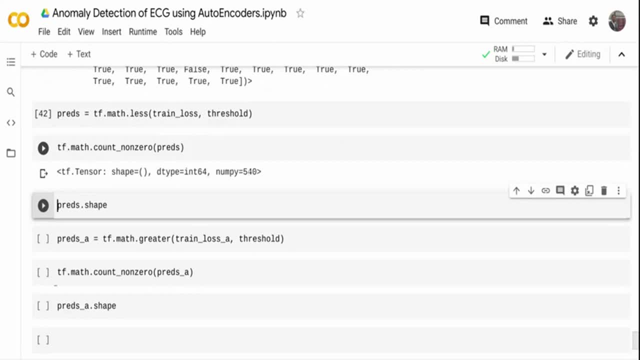 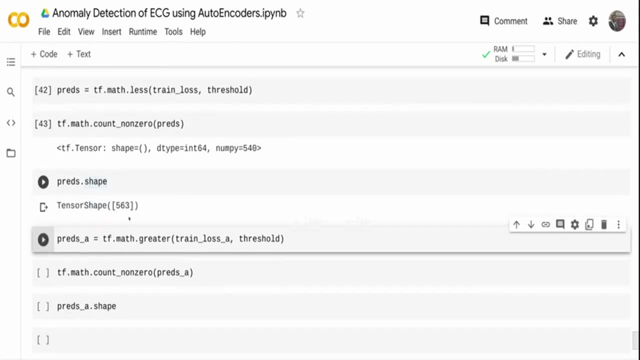 i'm checking what are less than the threshold, right, if 540 are predicted correctly and what is predicted it's around like of 563, right? so our model is almost, if you see, like 563 is the total value, 540 is predicted right at around 23 is predicted long. so in this case, if you really 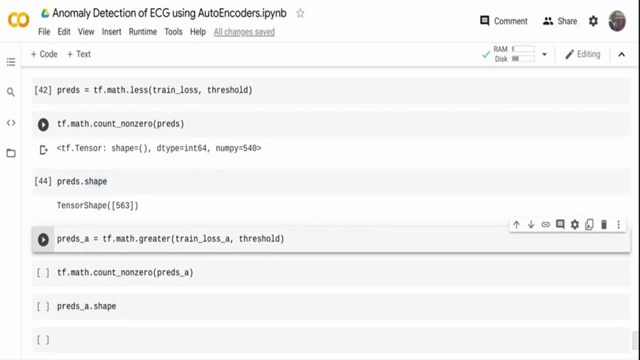 see our model is around like 95 to 96, accurate for the normal classes right now. let's go and check for the anomaly classes. now for anomaly, we need to find what is greater than the threshold right for the normal class. we found what is less than the threshold. in this case i'm using the greater. 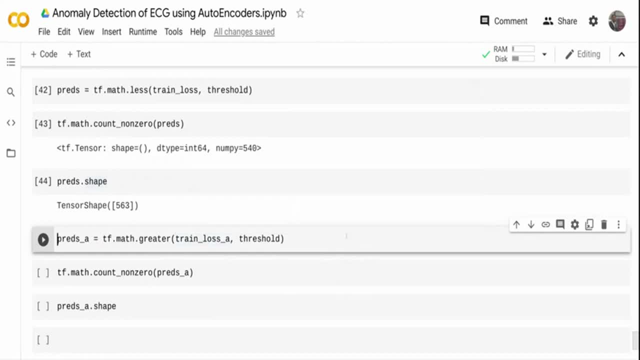 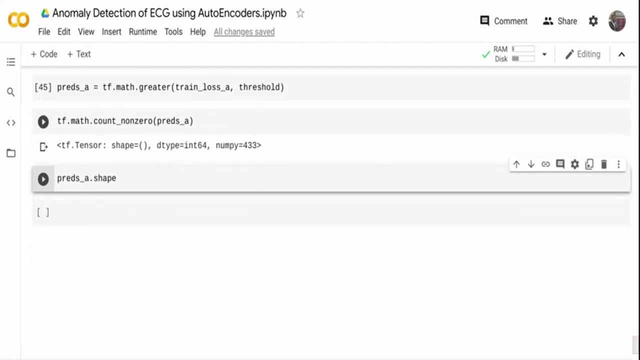 function and i am giving the anomaly class and the threshold right and it will give me the output predicted value and i'm counting the non-zero again of the predicted value in this case, if you see, it will tell us like: uh, 443 is predicted correctly. right, and what is the total? what is? 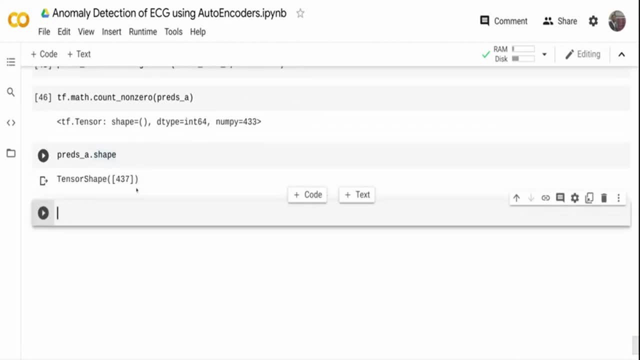 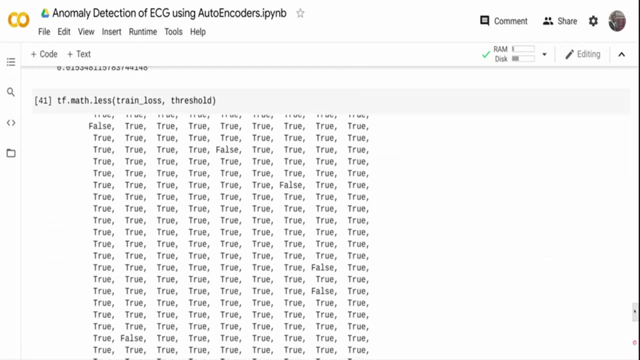 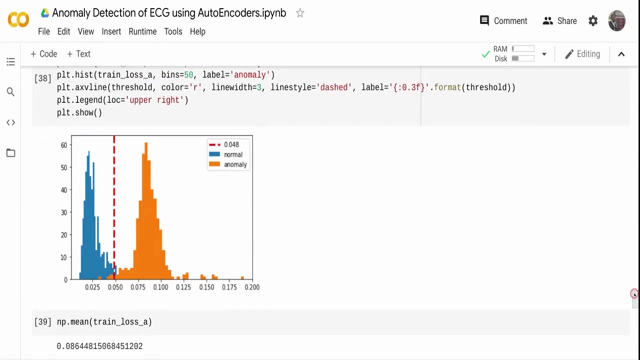 the actual shape of the predicted a. it is around 437. so basically, only four values were predicted. longly right, and that's what you're seeing over here on the top. uh, basically, these are all the four values that are in a orange color, that is below the threshold right, and that gives us a model which. 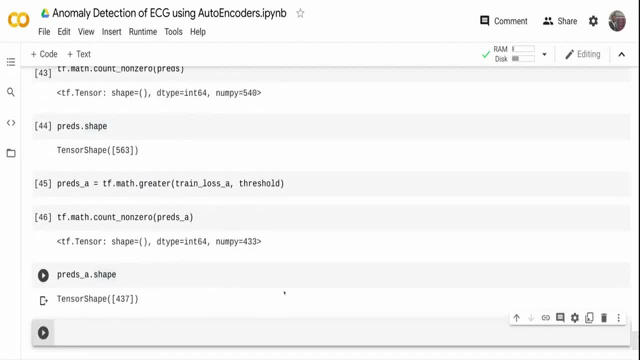 is able to, uh, predict like anomaly class almost more than 99 percent. uh right, if you do a simple math it's going to be more than 99 percent. so our model is able to predict anomalies more than 99 of the time, whereas the normal 95 percent of the time. now, according to your business object, you can 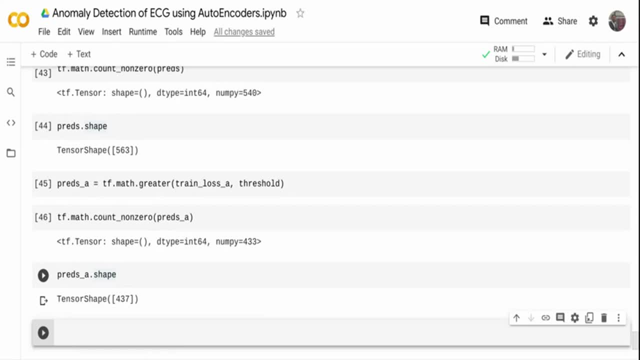 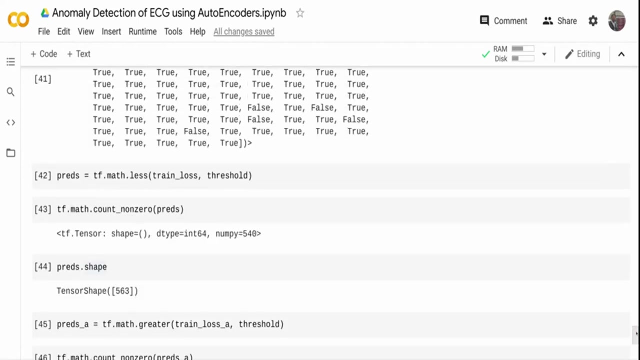 move the threshold so that the normal classes are predicted better than the anomaly classes. right wherever you move the threshold, the one class is going to benefit and other class is going to impact it. so this is how you build an anomaly detector using auto encoder. now you can use lstm. 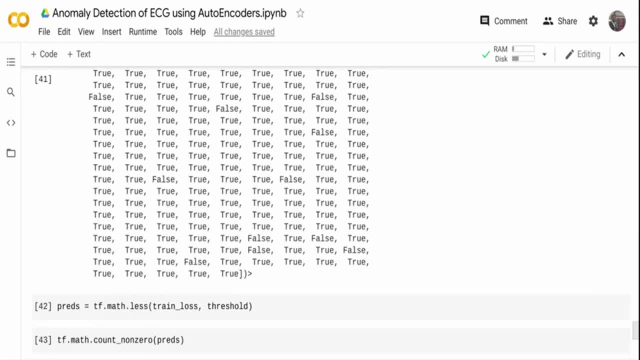 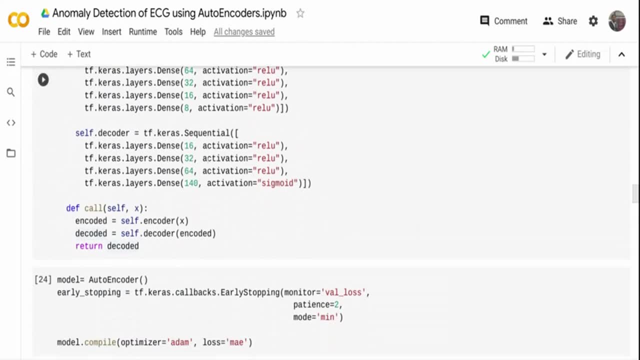 you can use convolution 1d. you can use lot of different architecture. so the architecture that you saw on the top over here, this can be any architecture. it can be an lstm architecture, it can be a convolution 1d architecture, but this is the base for everything. right? this is how you build.